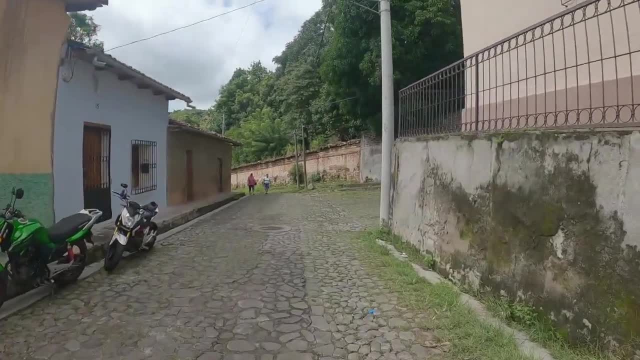 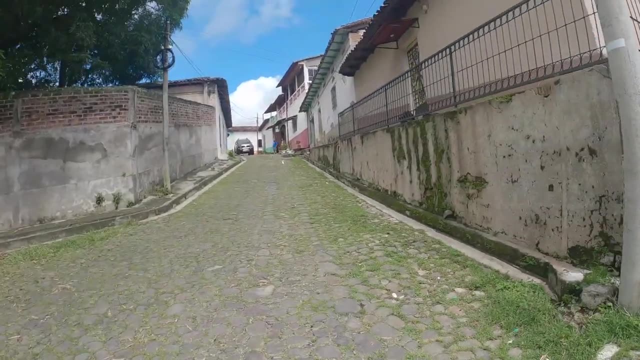 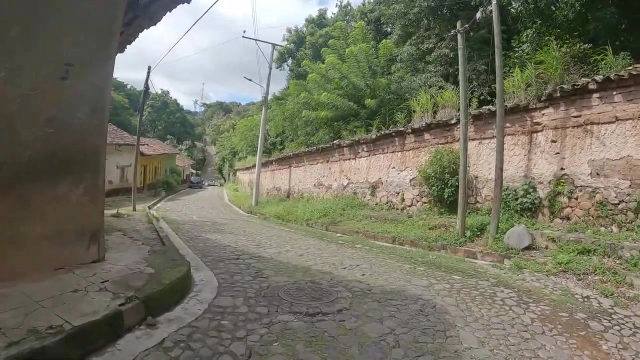 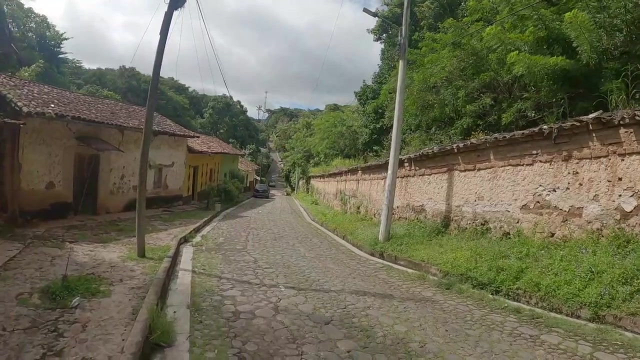 out, But join me to the bus stop Now. if I'm correct, I believe the bus that we're gonna be taking- Oh, look at the little chihuahuas- The bus here, Buenas, I believe the bus that we're gonna be taking is the 129, or the 129A, I believe. 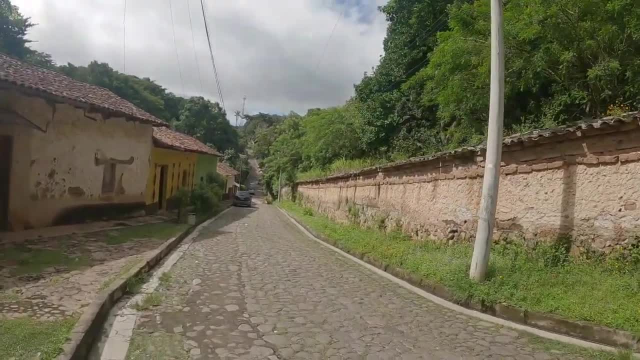 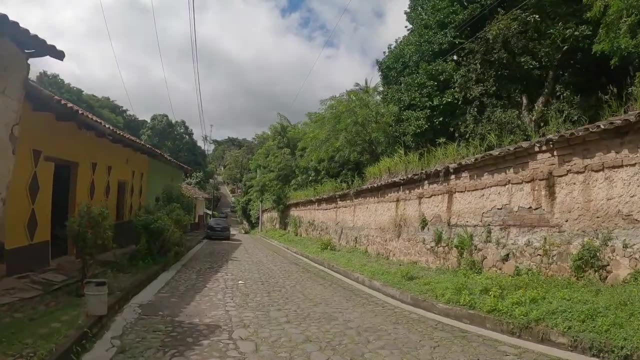 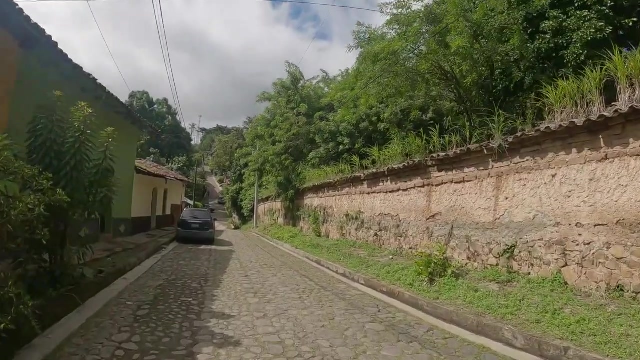 But, oh my gosh, look at this hill. Now I can say that it does look very beautiful and picturesque, though I love how plush El Salvador is. There's so many trees, There's so much nature. It really just gives this very clean and cozy vibe to it. 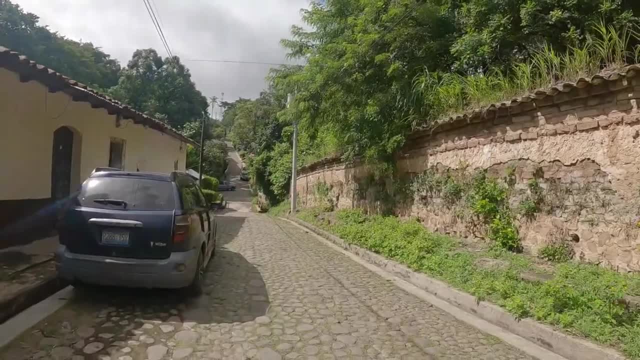 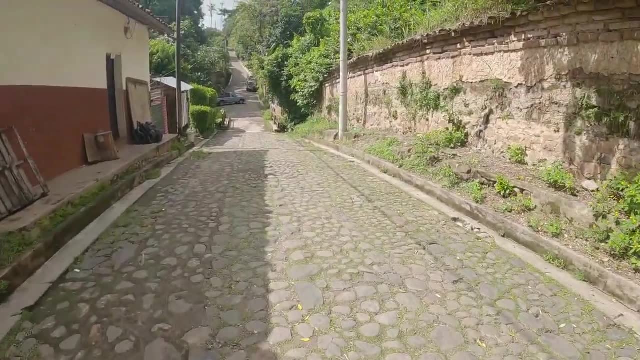 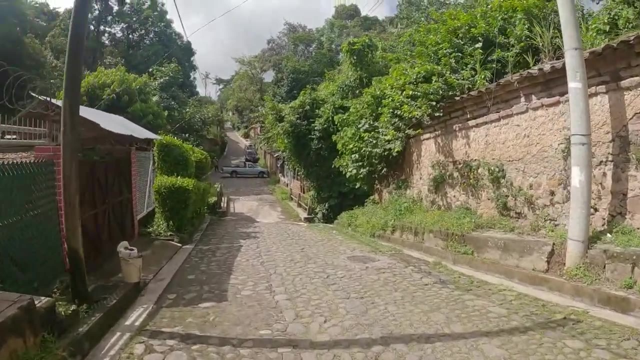 Oh man, Guys- I cannot stress this enough- Please wear some comfortable shoes. I'm steady, My foot is steady, getting caught in between some of these cobblestones and my ankle is like jeez. What is that out here? It's like a waterfall or something somewhere. Is this? 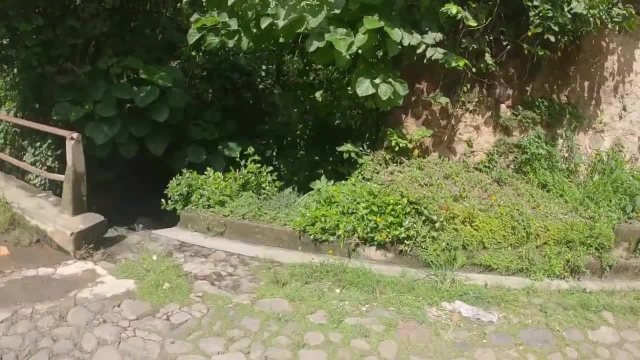 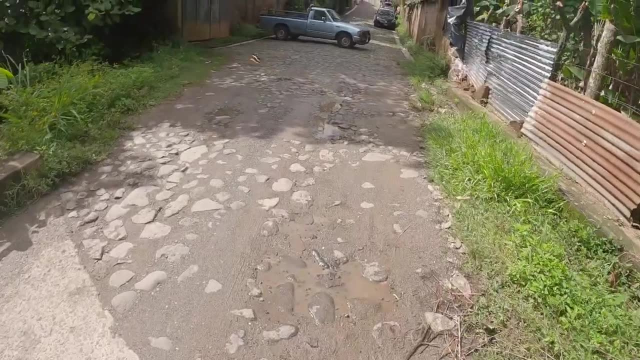 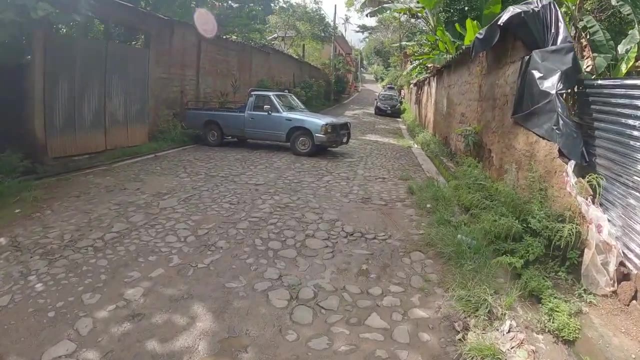 the river running through here. Oh yeah, it is Nice. It's flowing through there. Watch your step. Is he trying to turn around? You got it There you go, Buenas. I'm gonna try to get it. I'm gonna try to get it. 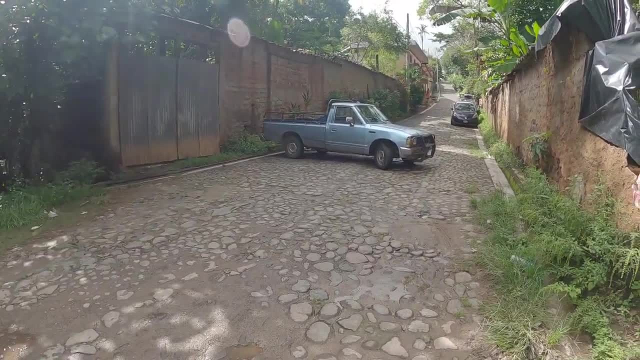 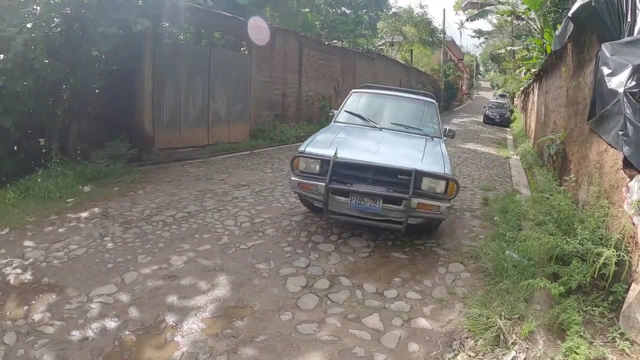 Oh my gosh, I'm gonna try to get it. Oh my gosh, I'm gonna try to get it. Oh my gosh, Oh my gosh, What is this? All right, That guy drives like my aunt. All right, Here we go. 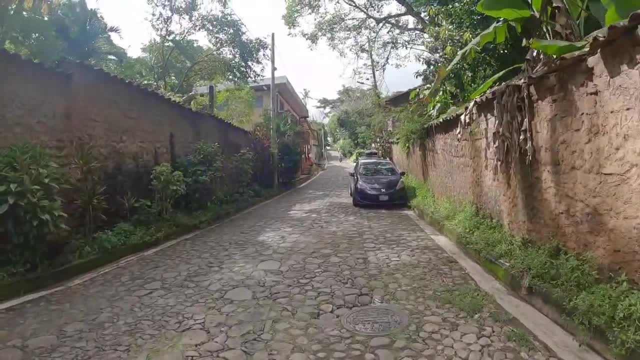 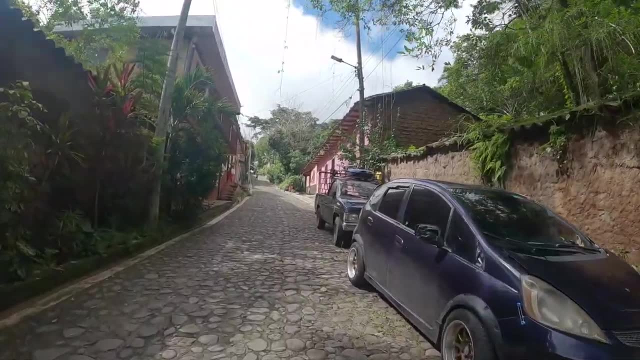 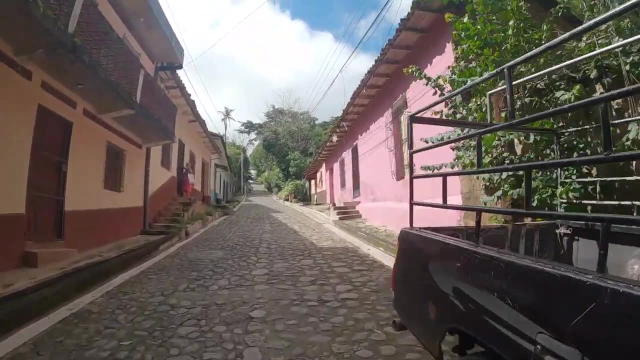 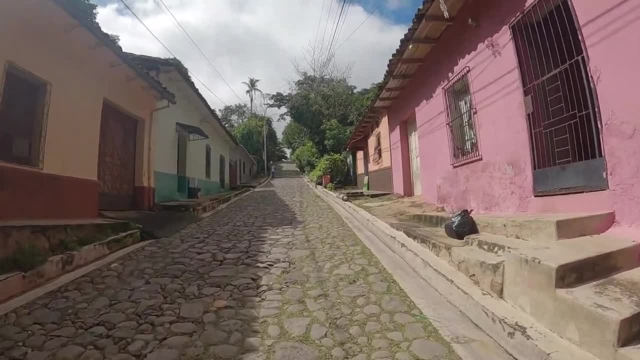 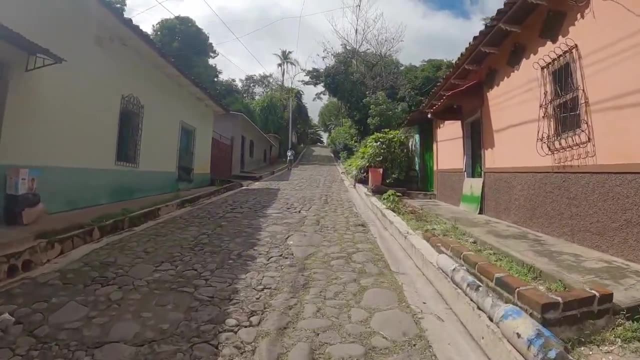 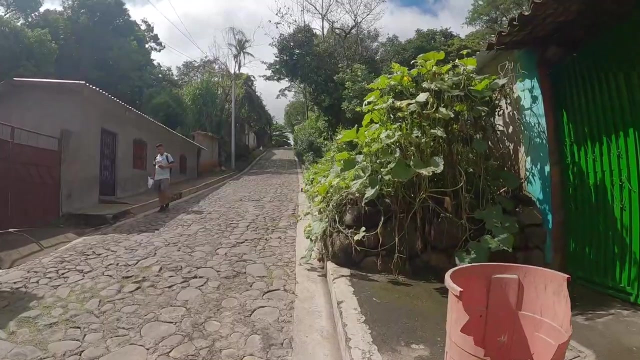 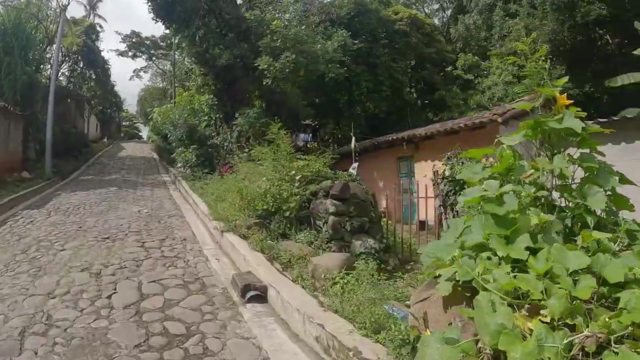 Buenos, Buenos, Buenos. All right, so I guess right now we're gonna, I guess the uh. we can use this time to answer some of the most asked questions that I've had since I've been here, Probably the number one. 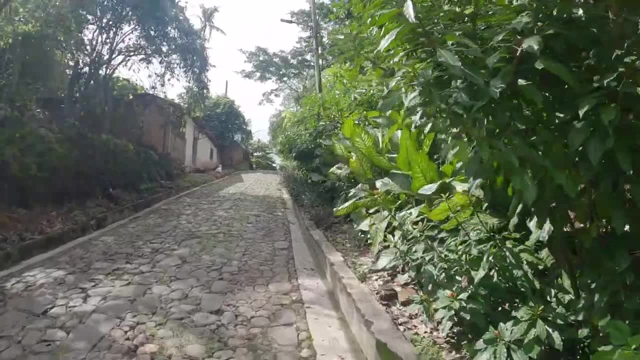 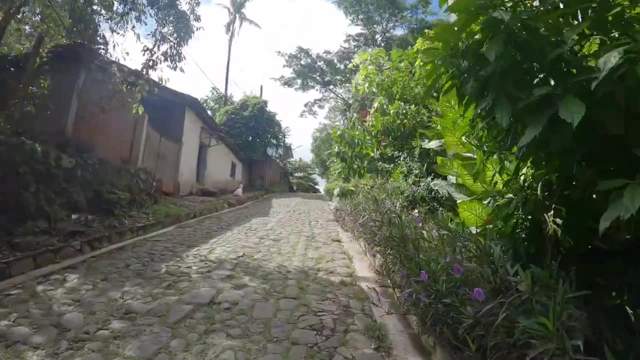 Ken, how's the nightlife? Definitely pretty good. I haven't really gone out as much, but El Tunco was definitely very good. and then I went out one night in. no, yeah, one night in San Salvador went to karaoke. That's gonna be in another video. 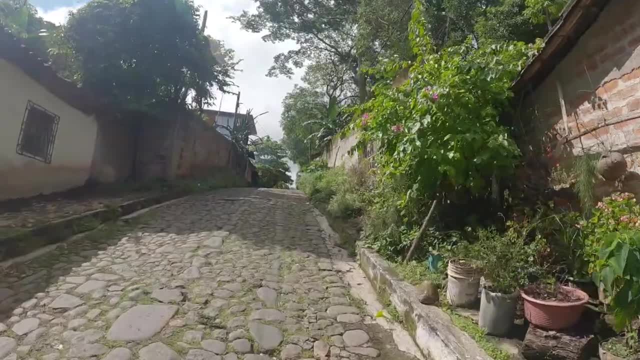 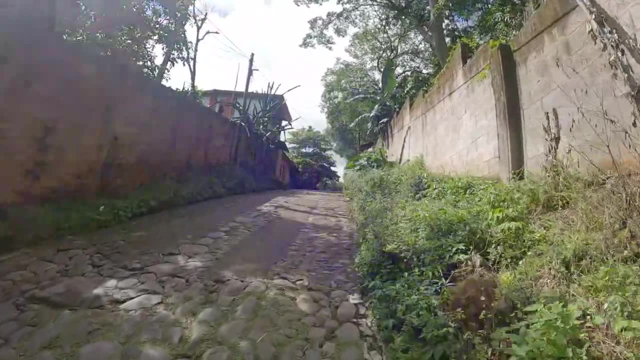 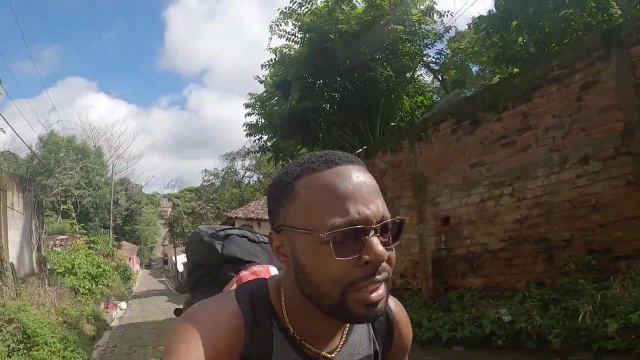 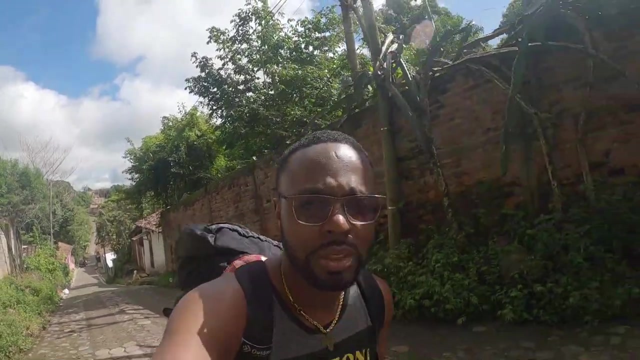 So today I was invited to a birthday party in San Salvador. If it wasn't for that, I actually would probably be going to Santa right now, or another city, So that's why I landed in San Salvador and then went to El Tunco and now Suchitoto. 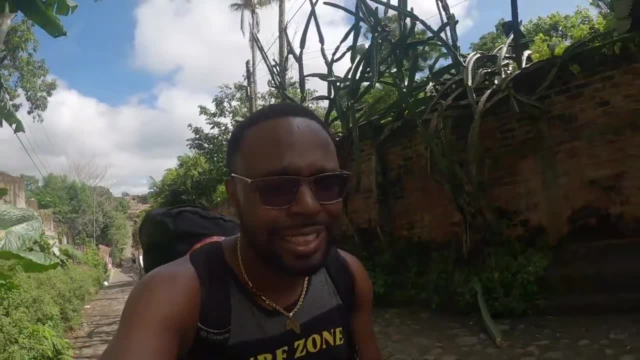 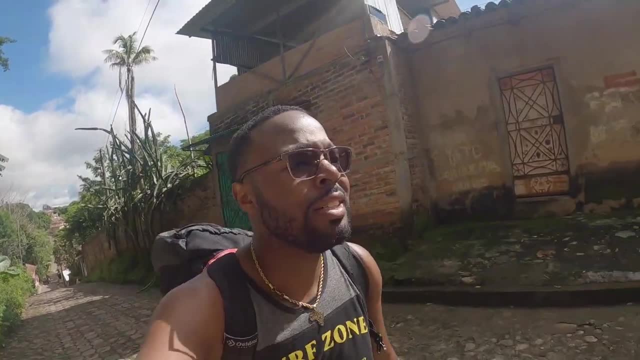 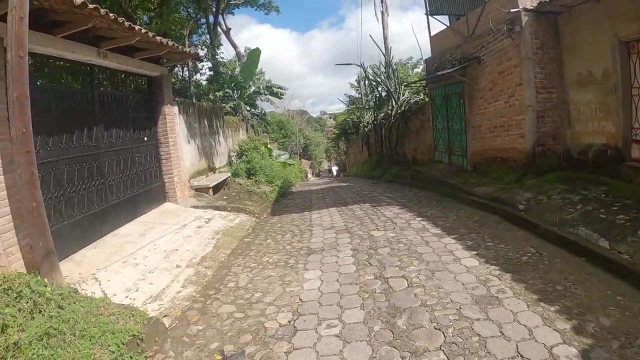 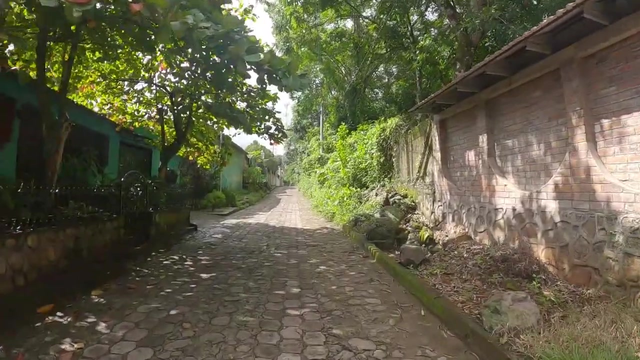 Now I'm going back to San Salvador, So I'm probably gonna stay in San Salvador for about two more days and then Thursday probably head to Santa Ana or another small town or village. Yo check out this hill. Y'all always talking trash, saying how out of shape I am, but that hill was steep yo. 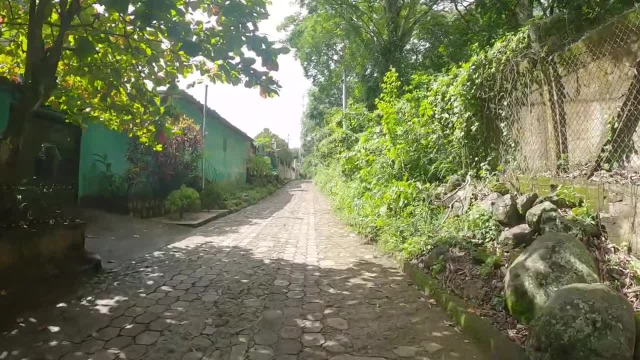 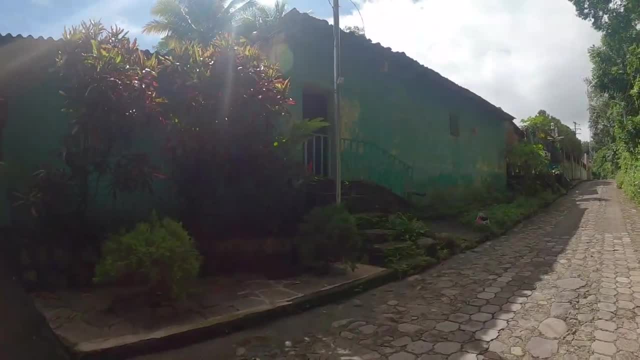 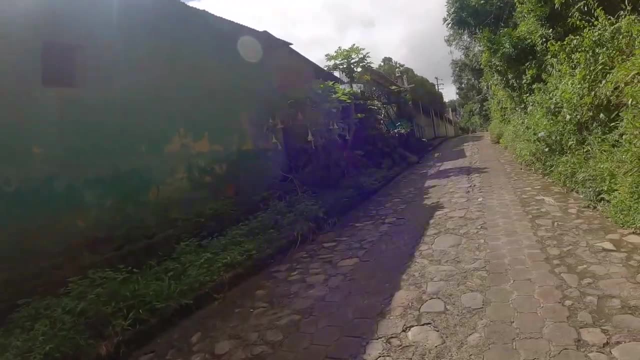 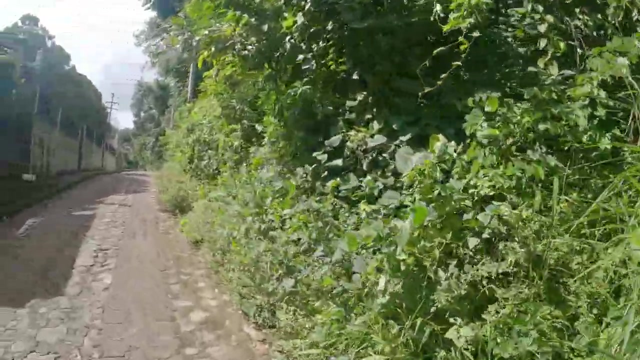 Okay, Let's keep going. So many of these homes here, just so beautiful. They've just kept their original um building artistic vibe and it just goes so well with the cobblestone streets and then with all of the trees and plushness of the nature. 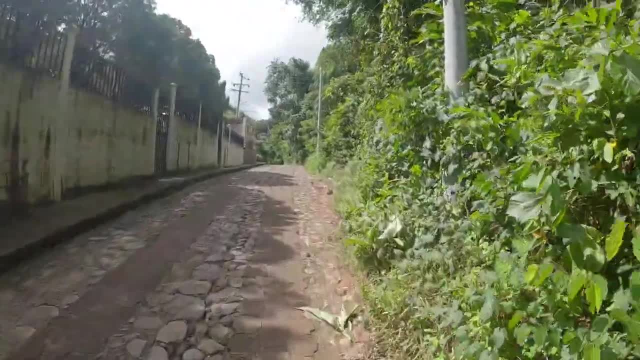 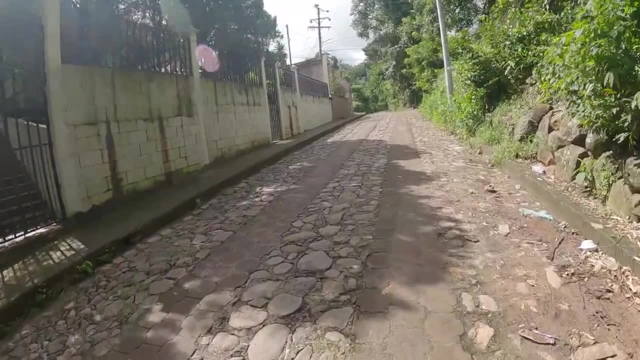 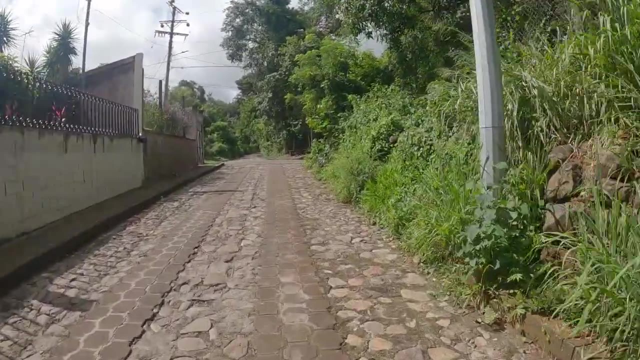 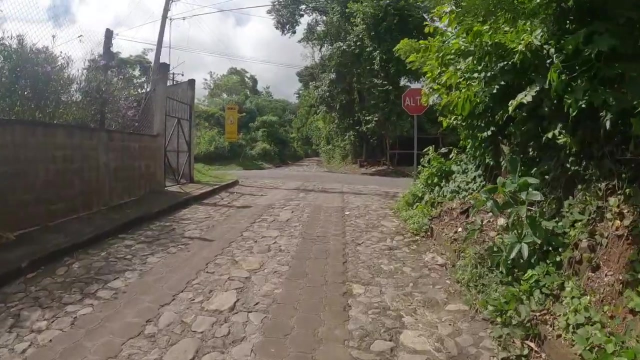 if you're in El Salvador, you have to make this uh a must stop for you all, right, okay, i think this is the main road right here and we're gonna make a right turn now. if you don't want to do the walk, if it's too late for you or 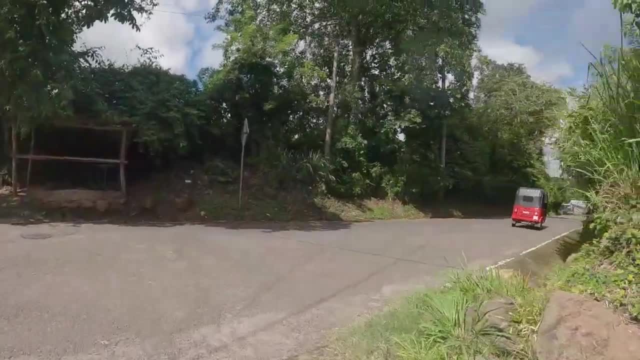 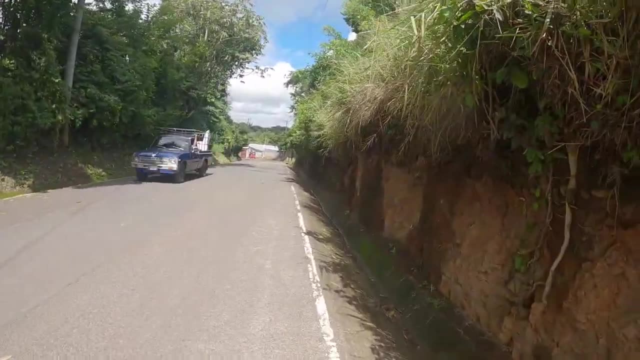 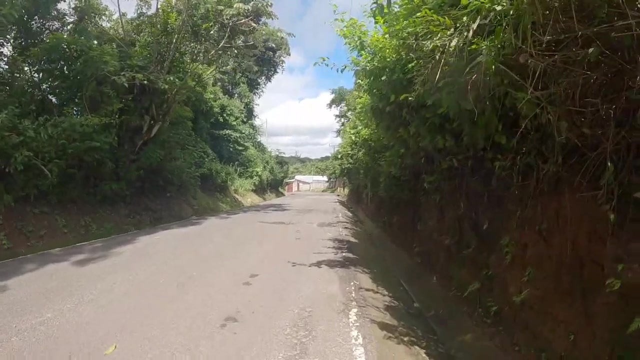 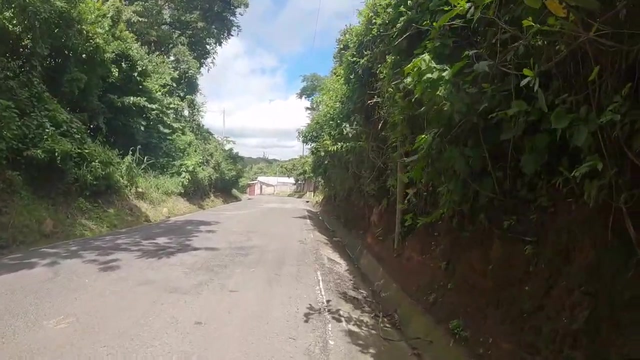 you're just not really comfortable doing it. you have tuk tuks and a little small moto taxis that you can take, but for me this is a good exercise for me, all right. i am very interested to see where i'm dropped off at in san salvador. 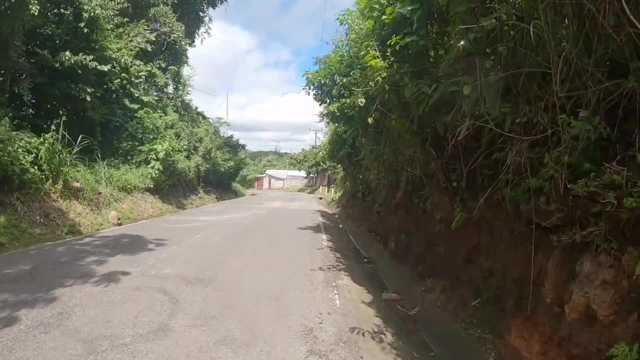 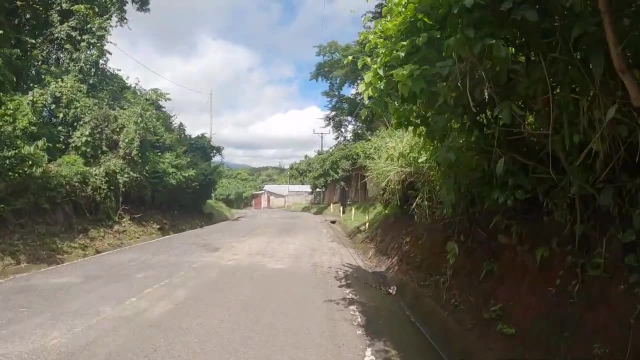 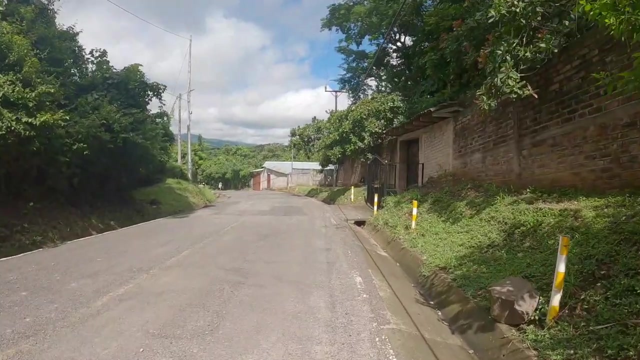 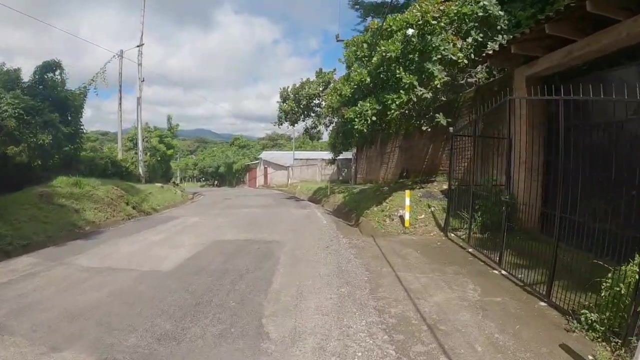 because i don't think it's going to be a traditional bus terminal. um. so as soon as we do get to san salvador, i have to ouch freaking bumblebees everywhere. as soon as we get to san salvador, i need to make a run to walmart and then i need to find a laundromat. 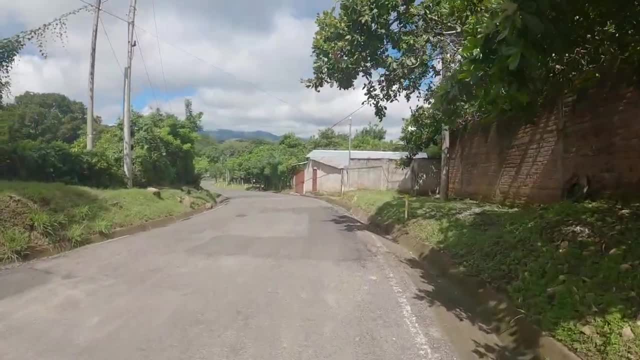 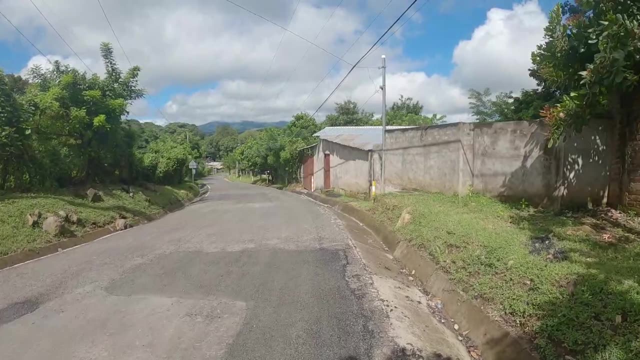 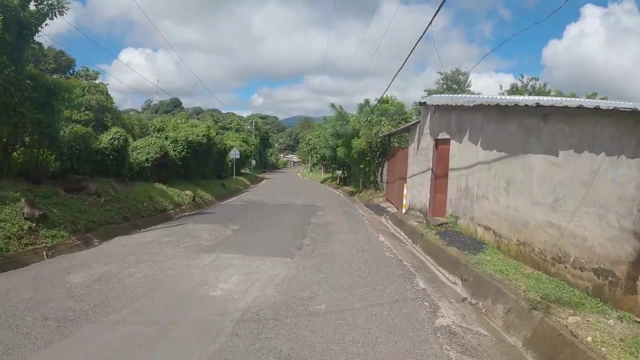 the airbnb that i booked. it is a guest house, but but it doesn't have a washing jar, so i need to wash and run a few errands and then we can get the day started all right. so i believe the bus stop is coming up, probably within a minute. should be coming up on the right somewhere. 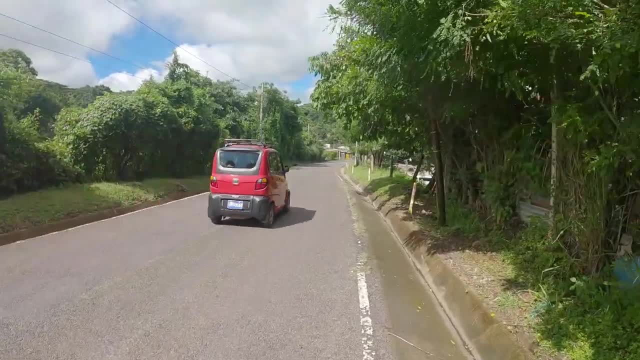 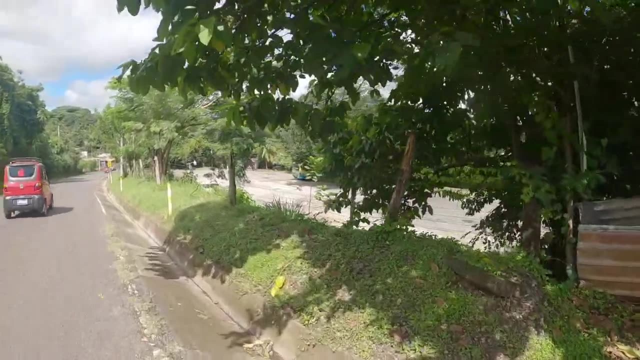 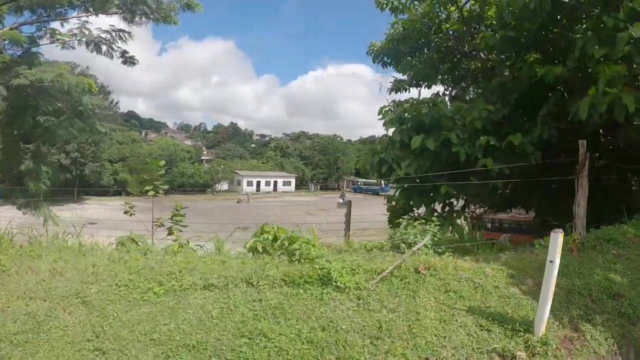 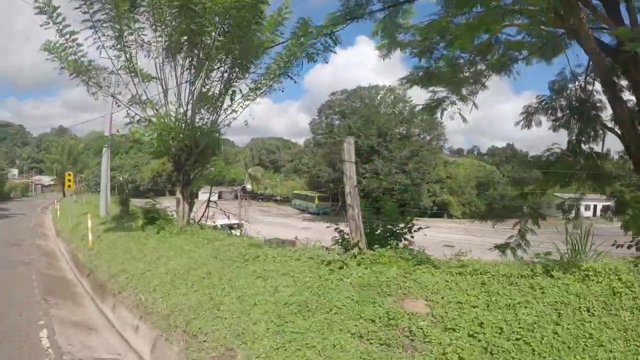 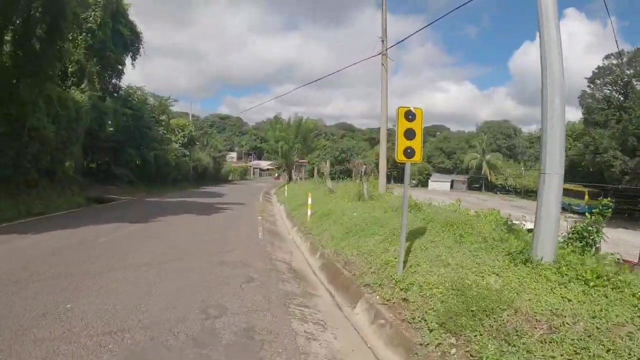 uh, is this it? i see a bus there. it says 129.. see, okay, well, that bus looks a little out of commission, though i hope this is the correct bus station. uh, so the the reception at the hotel said that the bus runs every 15 minutes. 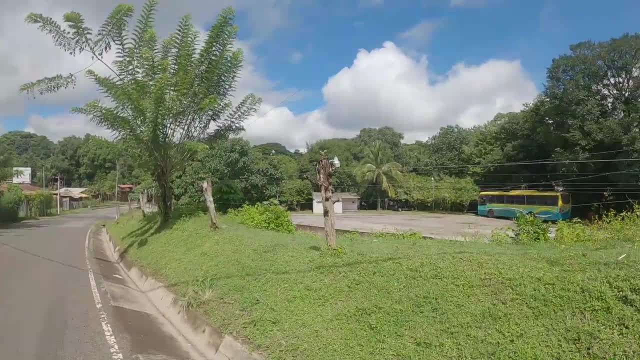 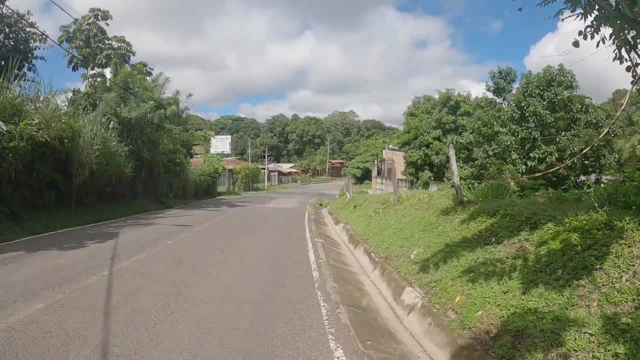 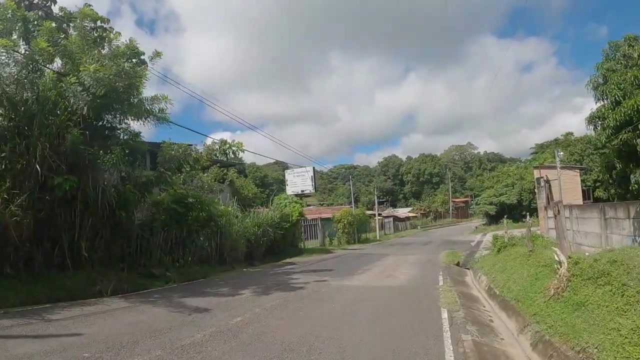 now i don't know if there's a place where i buy tickets, or do i just sit here and wait for another bus to pass by? but we're going to find out together. sala de recepcion beyond el mangal: fiestas, that's the only word i know. oh, baby showers nice. 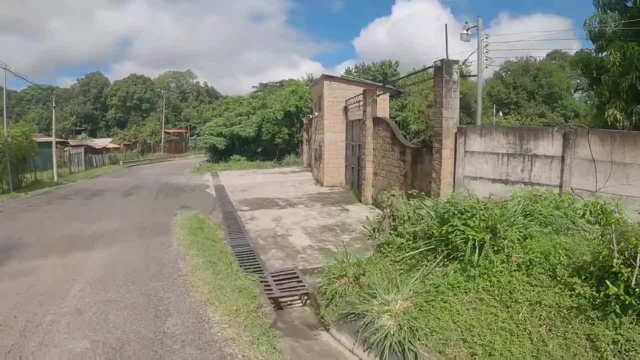 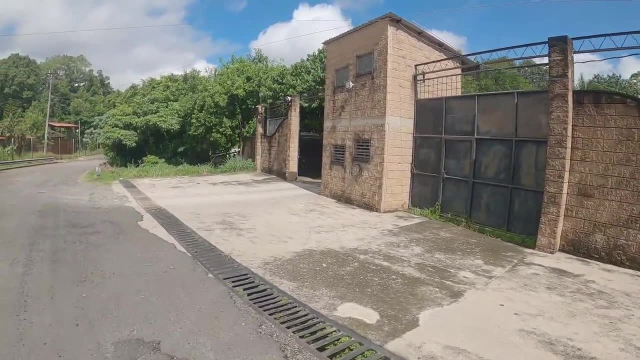 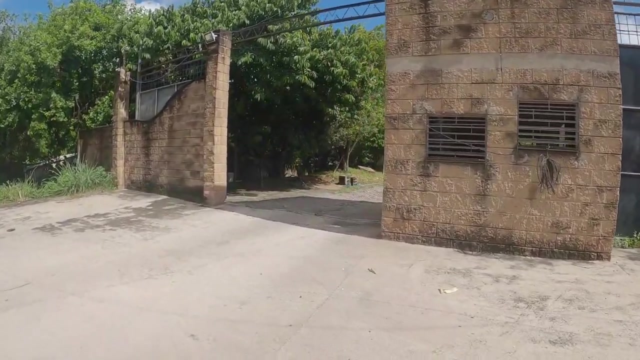 okay place to have events, all right. so i don't know if this is good or bad. this gate is closed, okay. this one is open, okay. i was about to say like it's closed. that would suck, guys. i cannot recommend this enough. please get a. um hello. 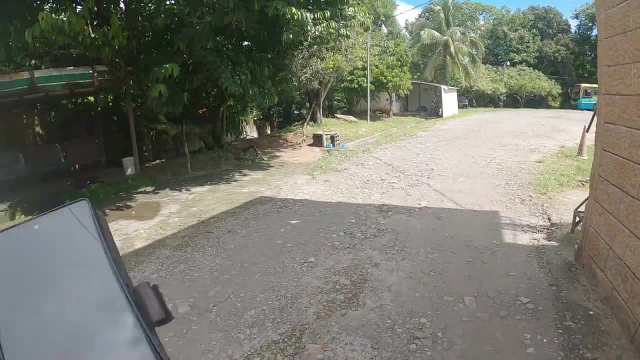 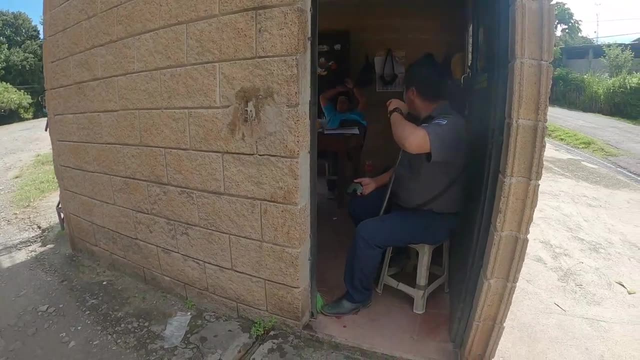 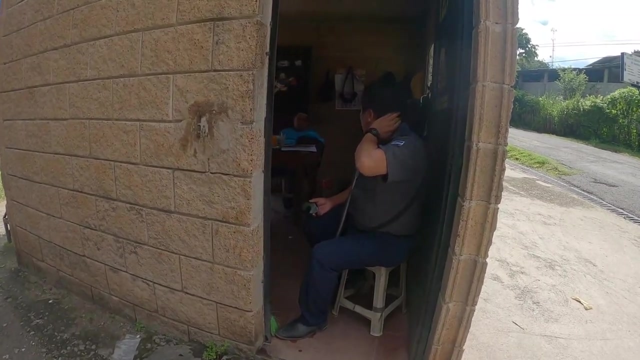 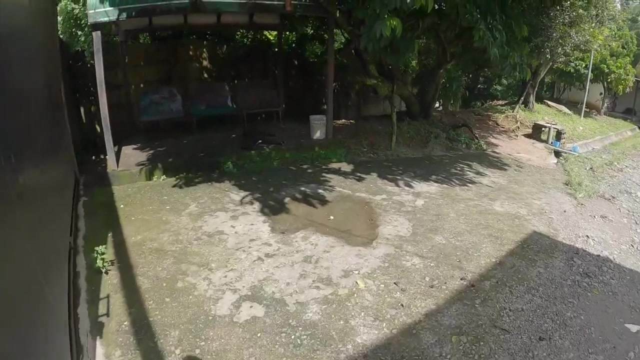 is this the bus station? oh, here, okay, what time is the bus? what time is it, i don't know? to san salvador, okay, to san salvador, okay. thank you very much. all right, guys, all right. look like it's raining a bit over here. 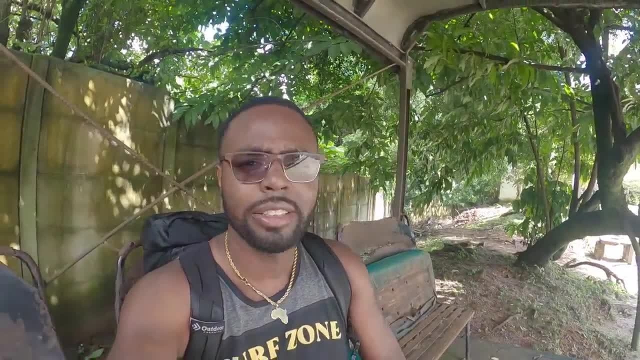 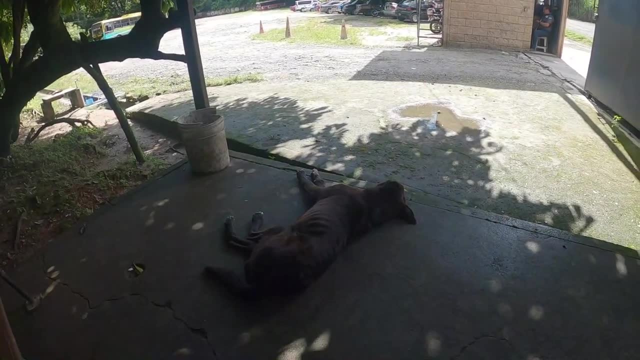 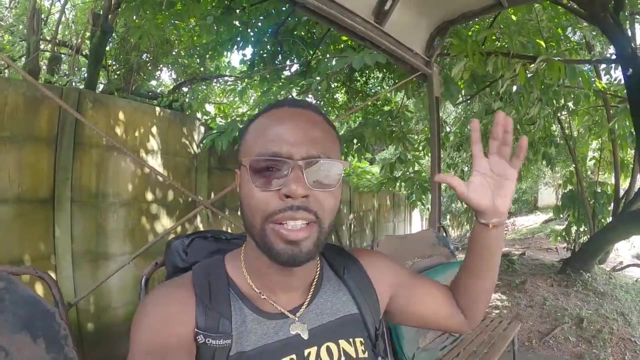 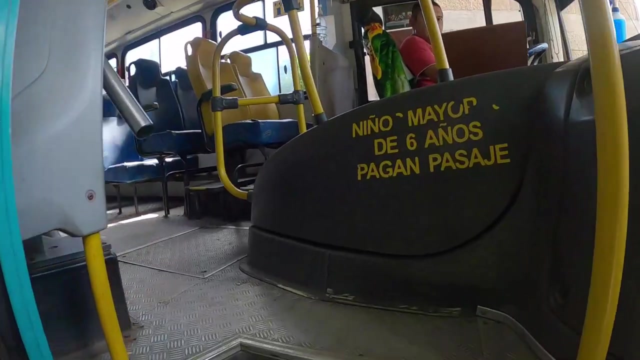 well, there you have it. that's the first part of this journey completed. now we're just going to sit here with her new friend here and wait for bus 129a to san salvador. let's do it, san salvador, how much one. thank you very much. 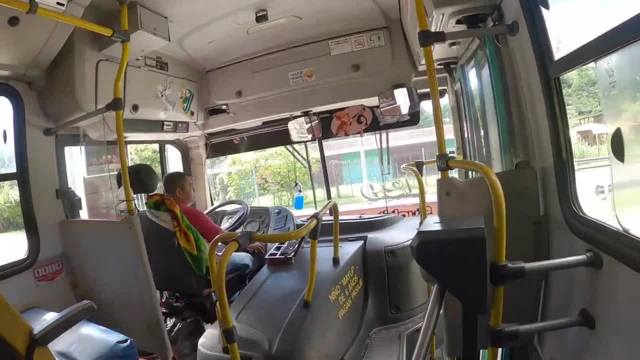 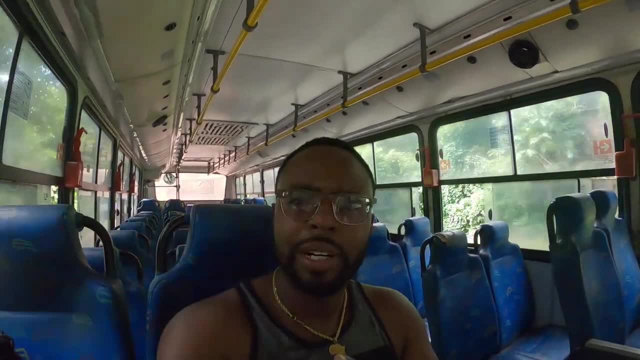 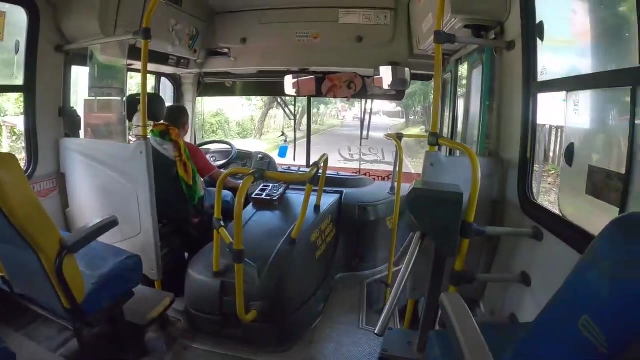 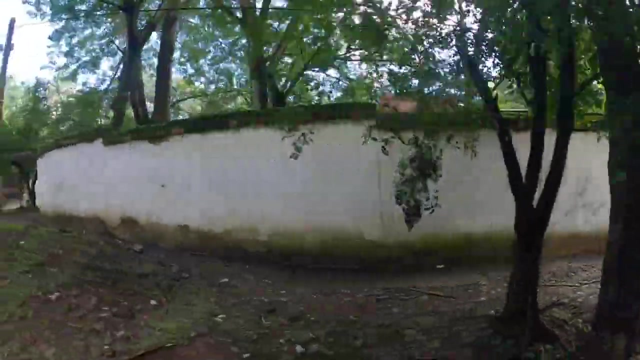 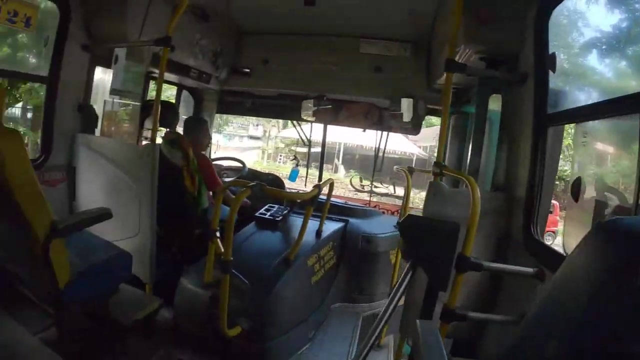 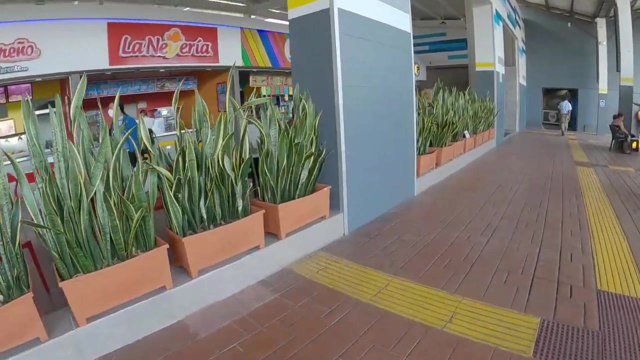 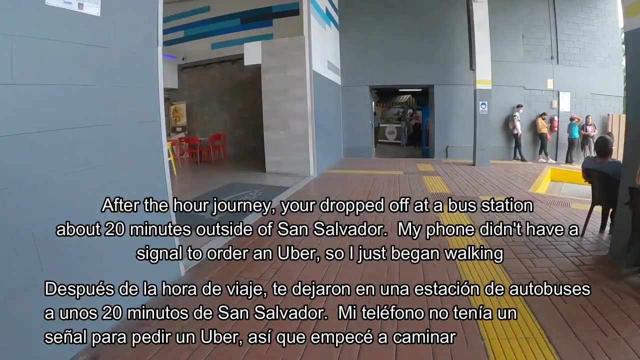 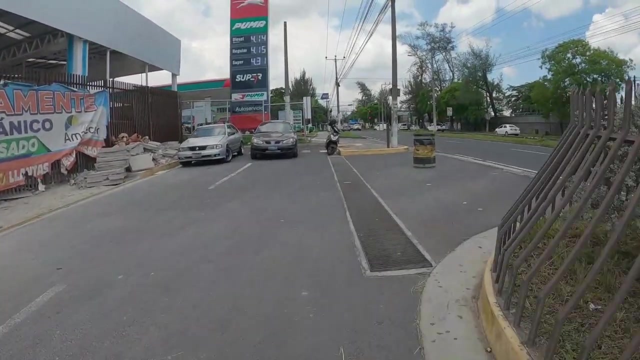 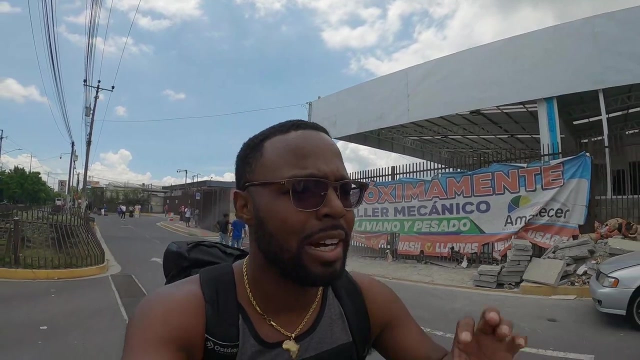 okay, there you go, guys. an hour ride from suchitoco to san salvador costs one dollar. amazing, wow, good, we're here. oh, oh, what a beautiful. uh, it's a, it's a beautiful. all right, guys. so there's probably about a 15 minute walk into san salvador. 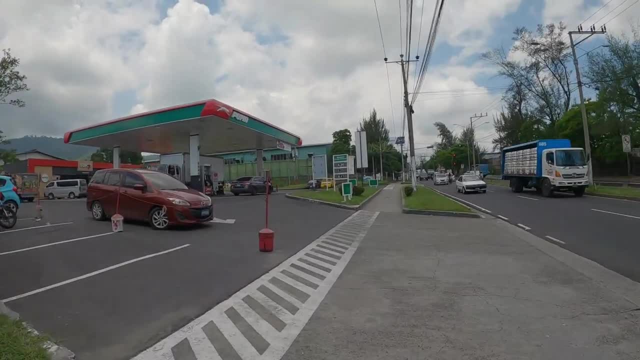 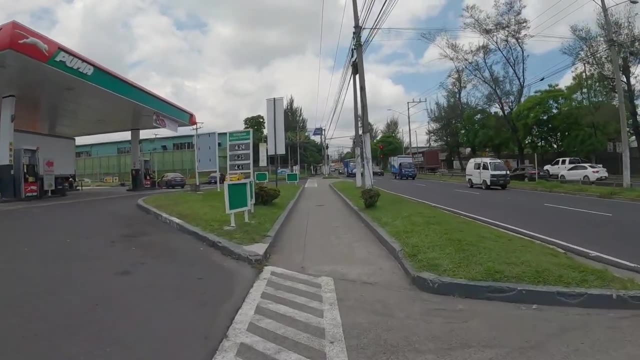 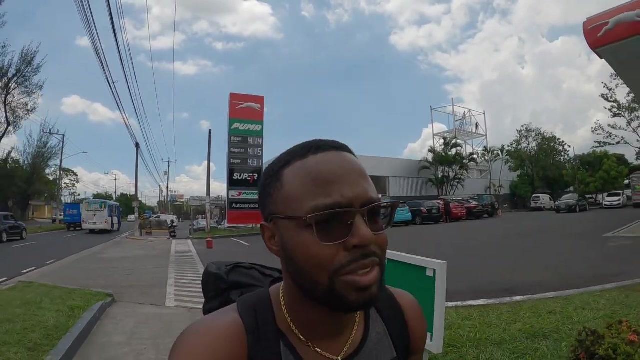 i'm not really for sure exactly, uh, where that bus terminal was, but we're just going to walk a little bit up the road here and see if we can get a signal so i can catch an uber. uh, i don't know exactly where the airbnb is, so 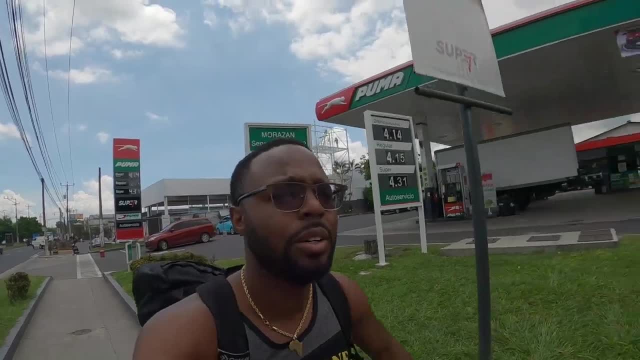 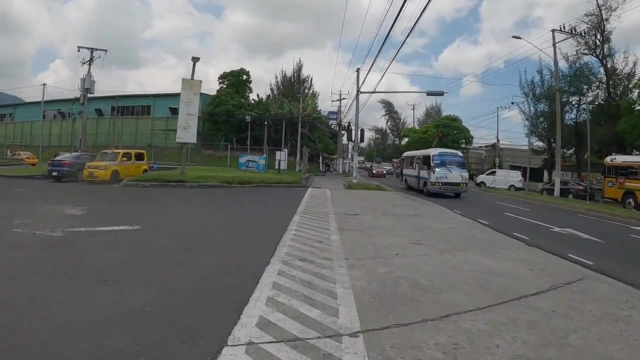 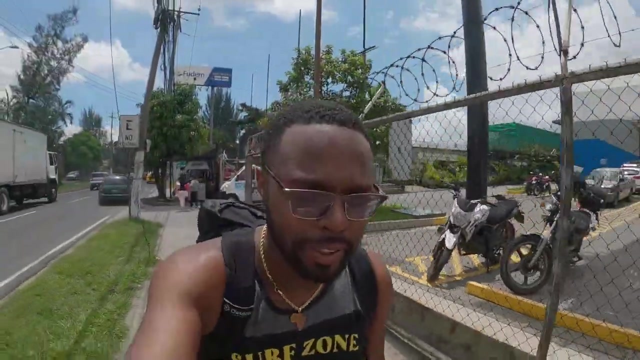 so next thing i'm looking for, i need a signal, so let's just keep walking. i'll tell you one thing: that food smells so freaking. good guys, the number one piece of advice i can give you if you're traveling to salvador, get a sim card right now. i'm completely 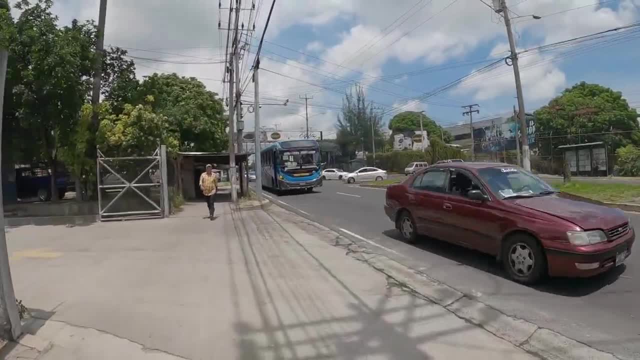 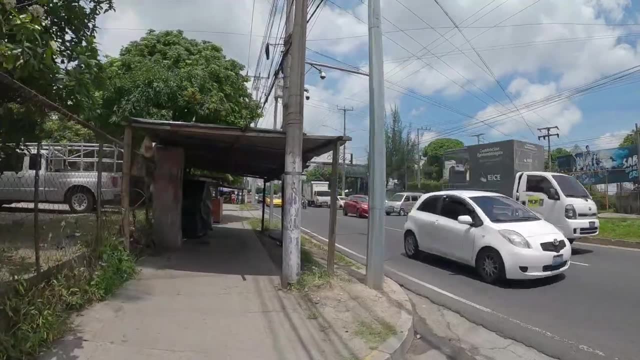 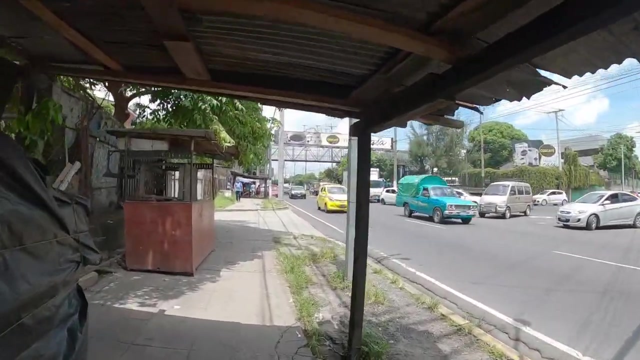 stout, so can't use gps or uber or anything right now because i don't have any signal. so the game plan: we're just going to continue to walk until i find some type of restaurant or anything that has wi-fi so that we can get to where we need to go. 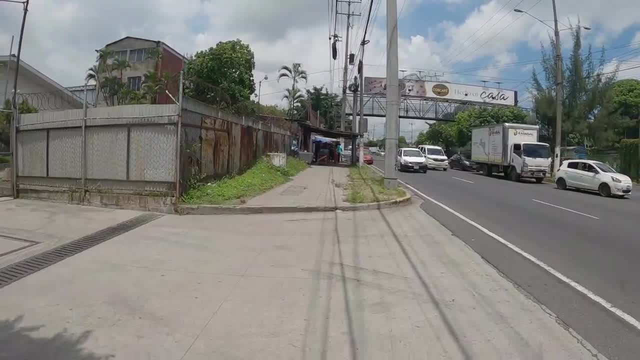 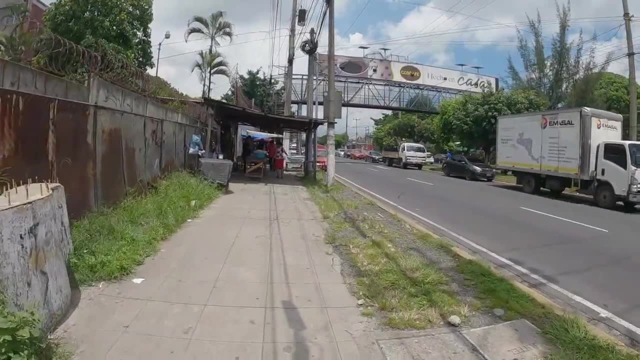 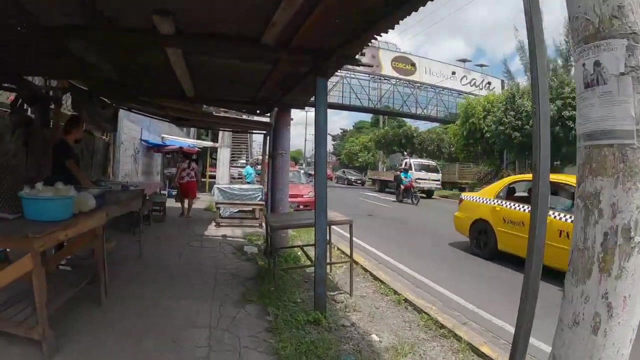 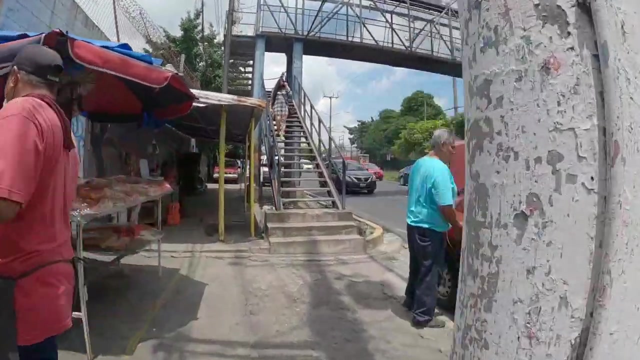 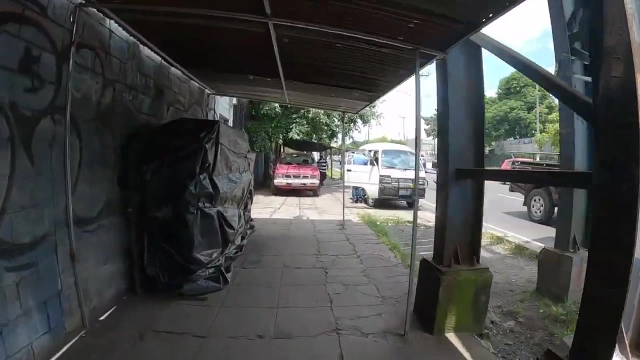 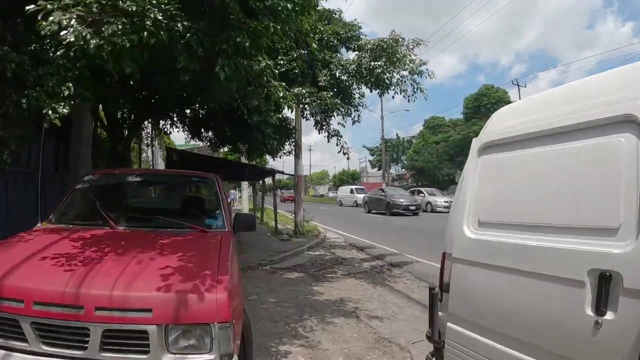 but in the meantime i am enjoying the journey. buenas, so friendly. it's up on the road. oh my gosh, the driving here is insane. oh, that looks good. i haven't eaten yet, and so it's kind of kicking in a little bit. i can feel my energy reserves kicking in. 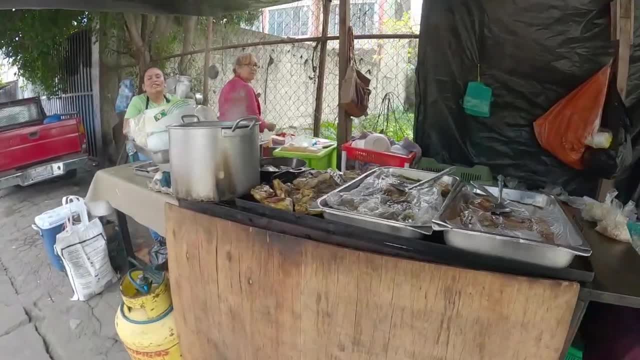 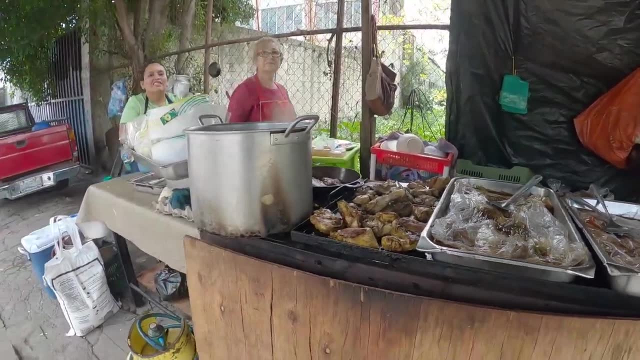 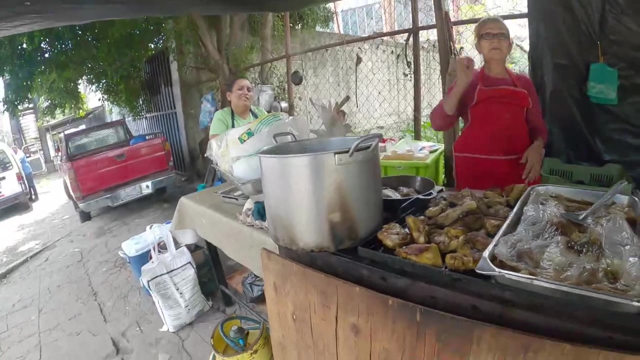 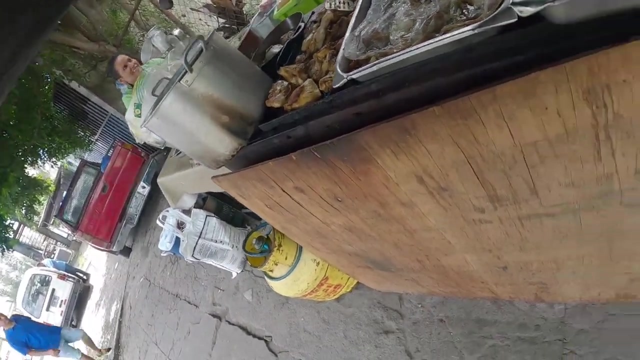 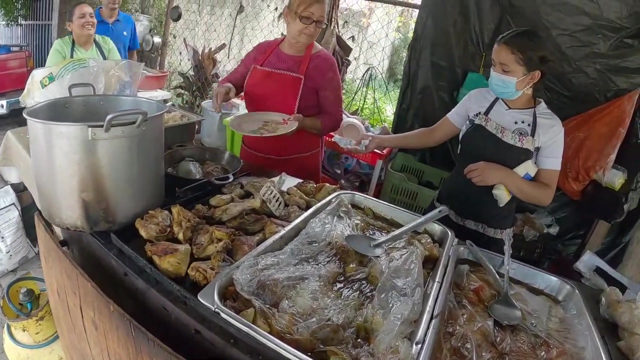 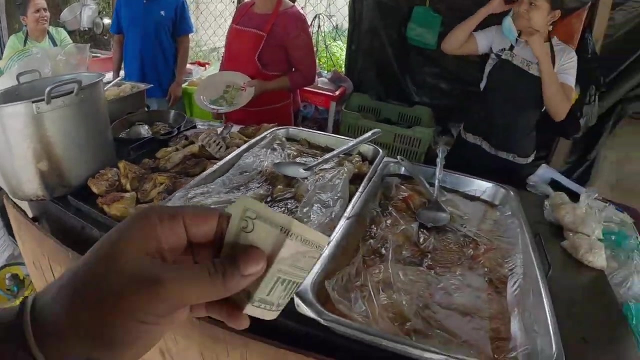 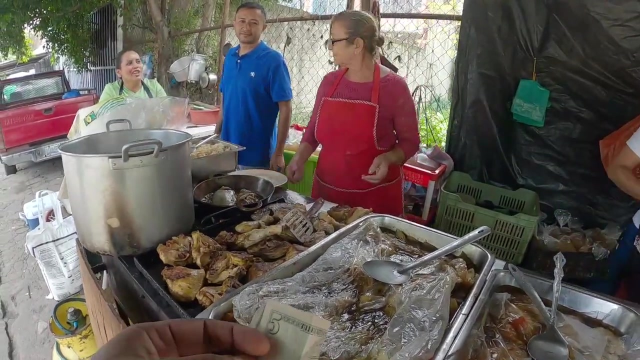 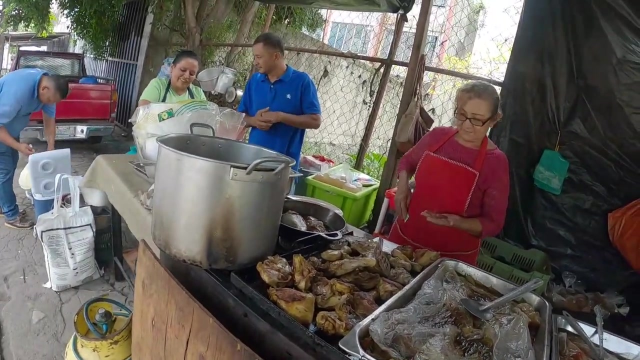 oh, that looks so good. hola, eh, cuánto uno, oh dos, okay, uno por favor. uh, let's see how much. that's a half. ah, aquí, por favor, cuánto up to you, or no, tres, tres, no tiene que me lo cante. 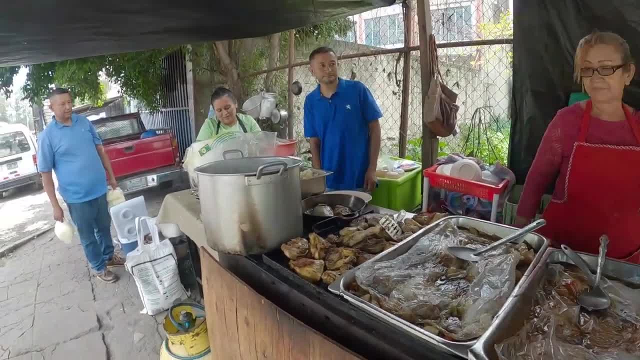 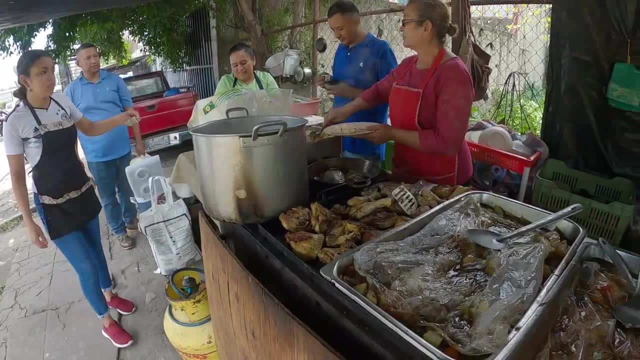 no tiene que me lo cante, voy a cambiármelo. ya se lo sirvo para comer aquí, okay, bien, okay, no está muy mojado ahí, no está muy mojado ahí. mejor allá en el carro póngalo. mejor allá en el carro póngalo. 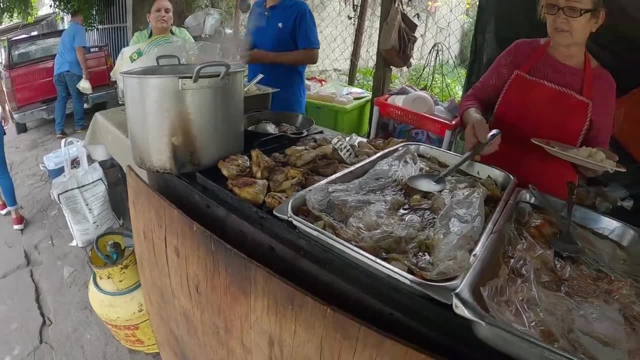 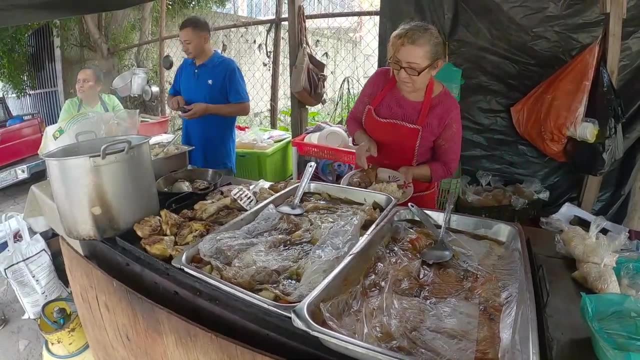 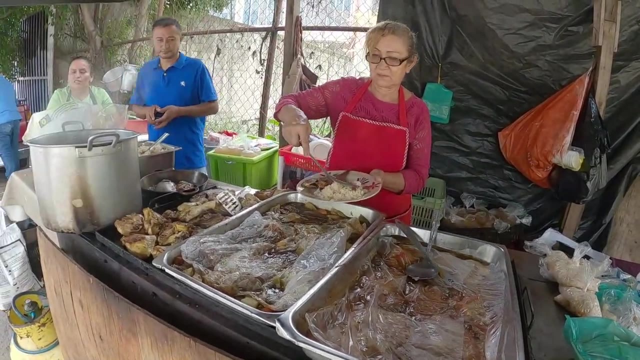 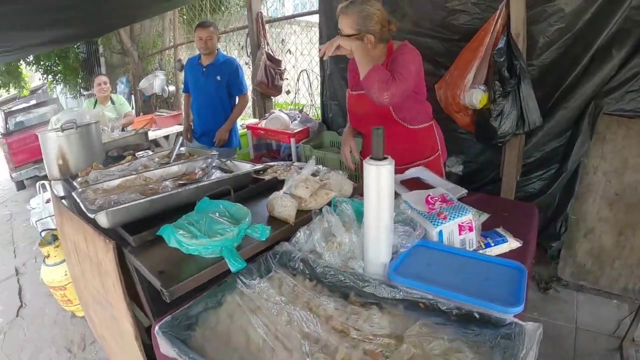 que le pongo pollo o carne, ah, pescado, carne, si pescado, si pescado. si le doy jugo, si le voy a poner queso, porque la ensalada, ensalada que todavía no tiene la mayonesa. 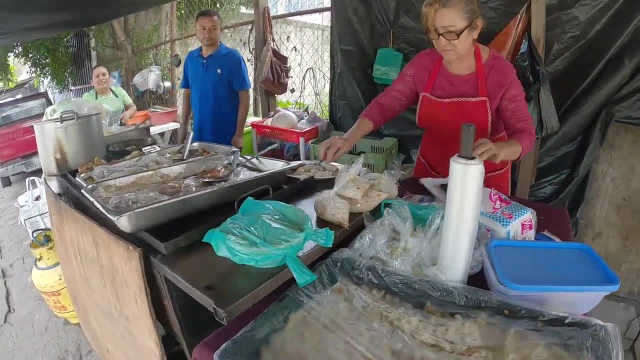 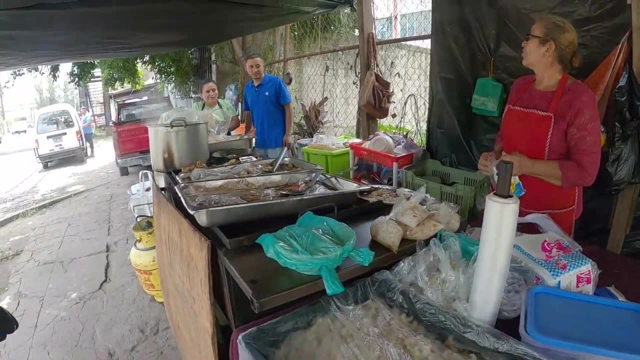 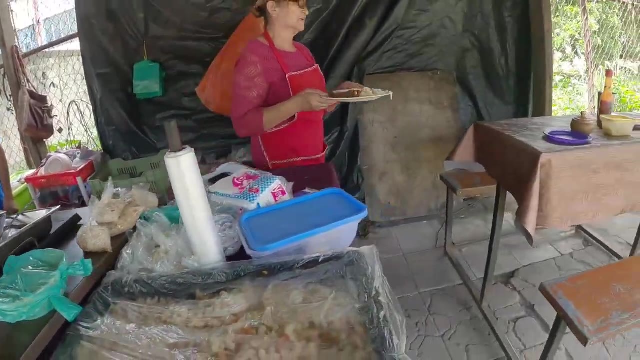 si le pongo queso, porque la ensalada no tiene la mayonesa. si le pongo queso, ah, no queso. si le pongo queso, no queso. i need water, comer, comer algo, comer pesado, pesado o tal comer pesado. 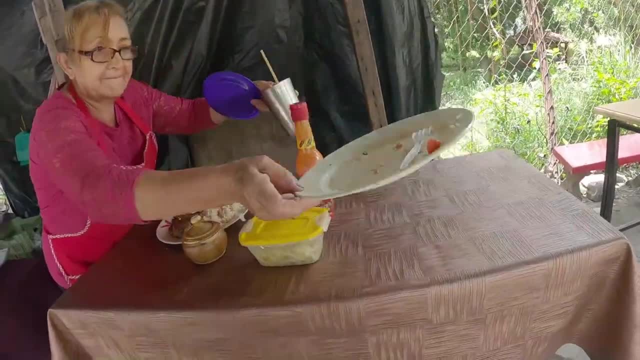 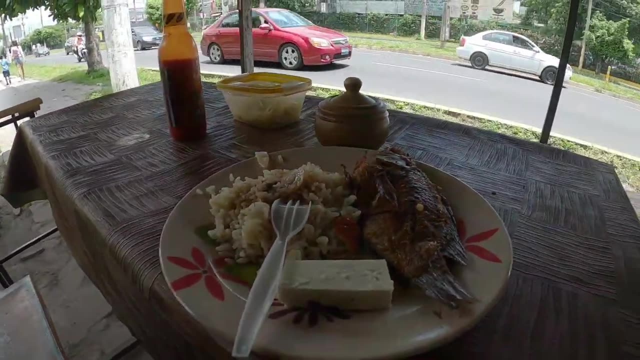 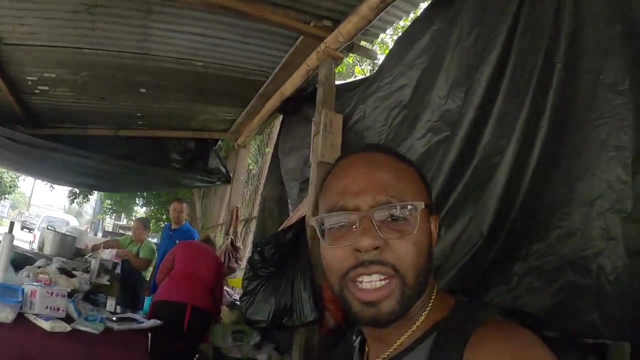 si, muchas gracias, si, muchas gracias, i'm gonna sit over here. i'm gonna sit over here, okay guys, okay guys, okay guys. we got some pescado with some arroz. we got some pescado with some arroz and some queso. all right, let's try some of this street. 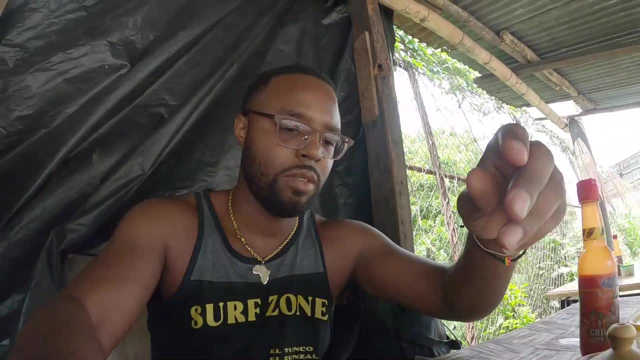 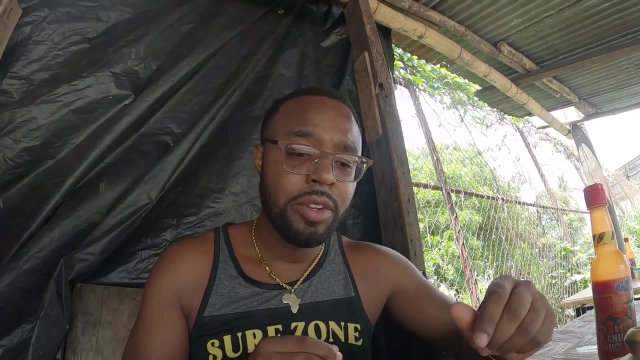 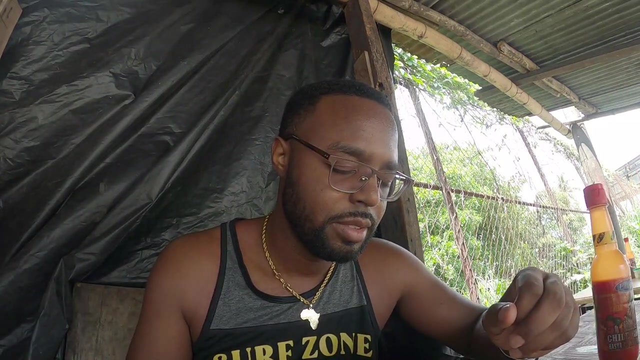 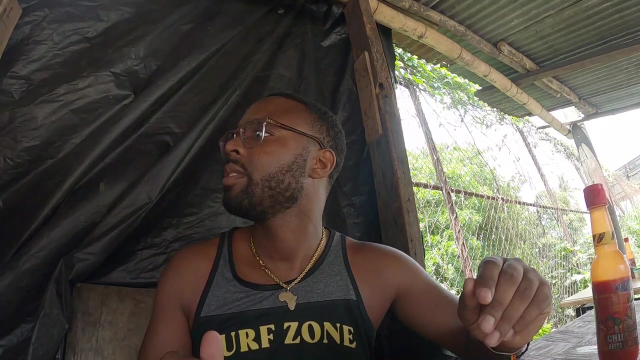 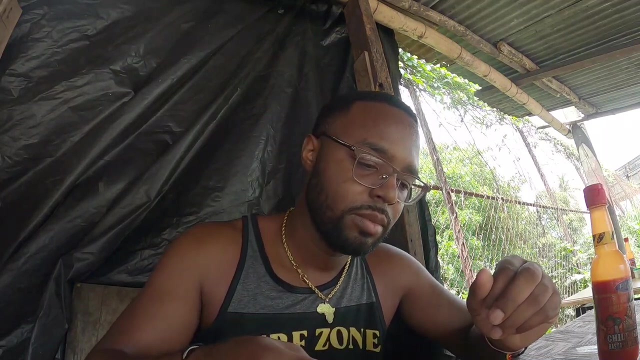 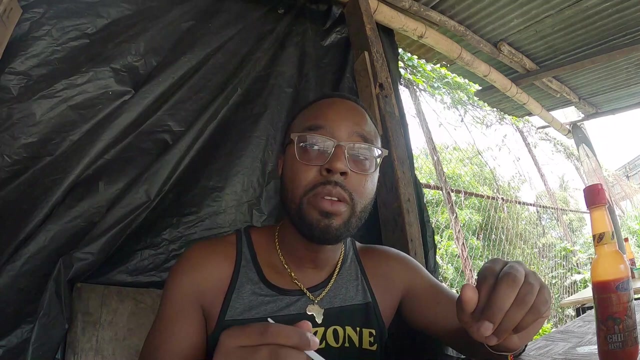 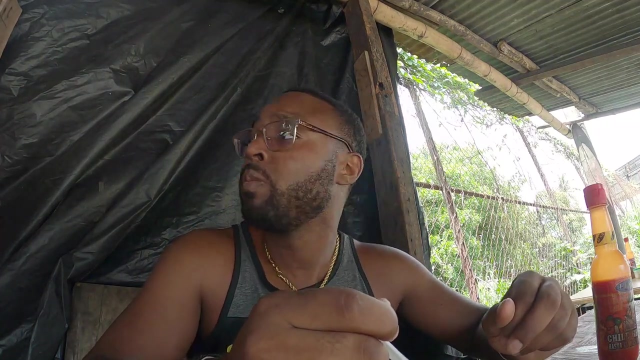 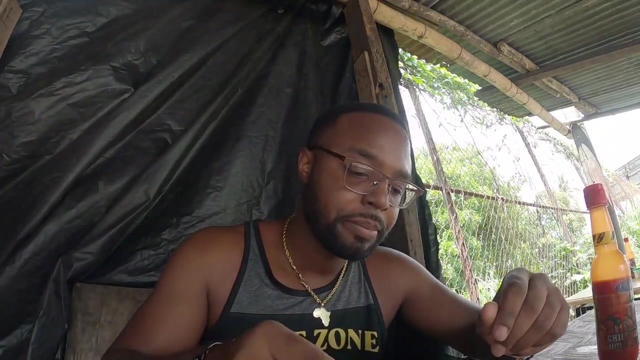 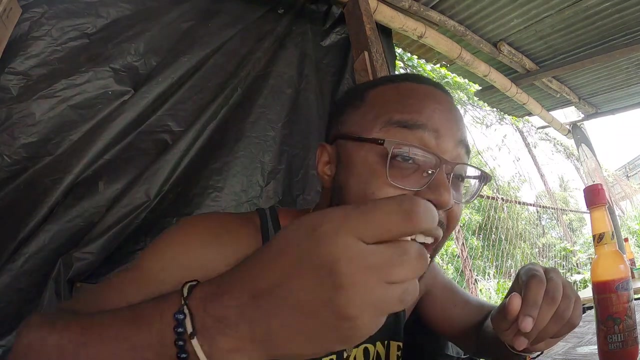 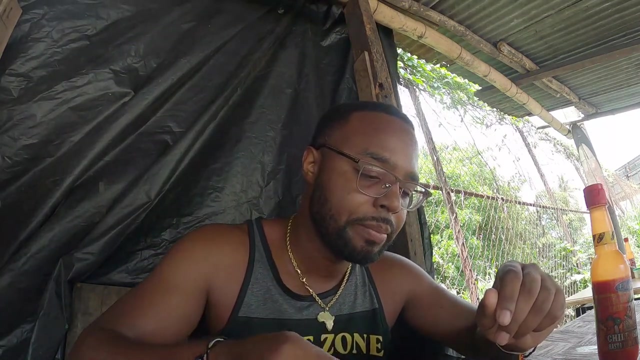 all right, let's try some of this street salvadorian food. all right, i'm excited to try this. uh uh, i'll say pan, pan, pan, pan, uh uh uh, Tejas, Tejas, Si, Oh God, that is very good. Alright, guys, as you can see, I've completely cleared my plate. 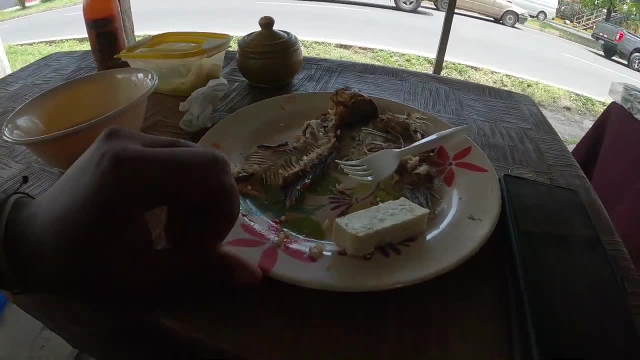 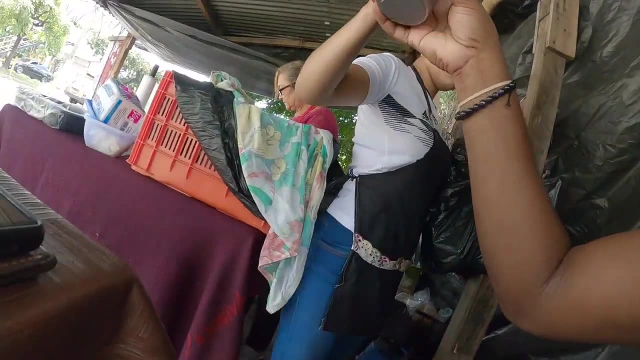 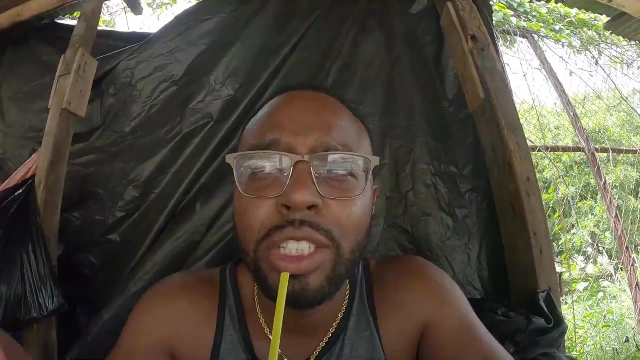 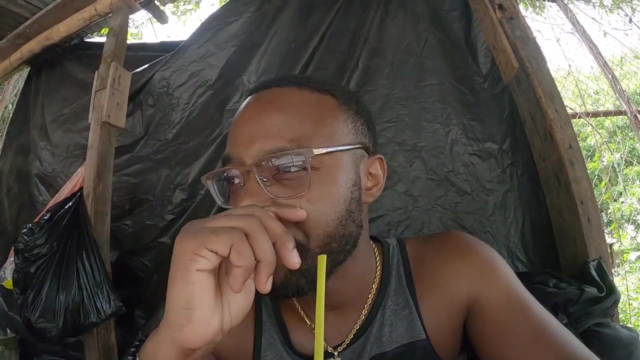 That was divine. Oh, I love street food, man. Alright, I just ordered a quick fresca and I'm going to get back to walking. Muchas gracias, Tastes like some apple juice and strawberry juice. It's very good. Alright, so the game plan. let's get back to walking. 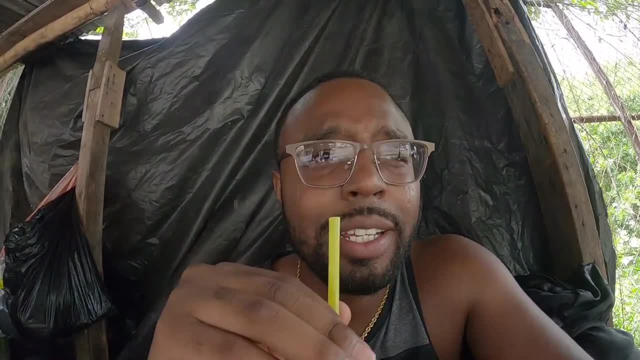 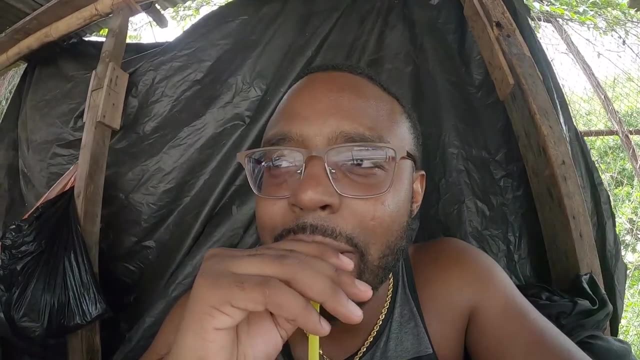 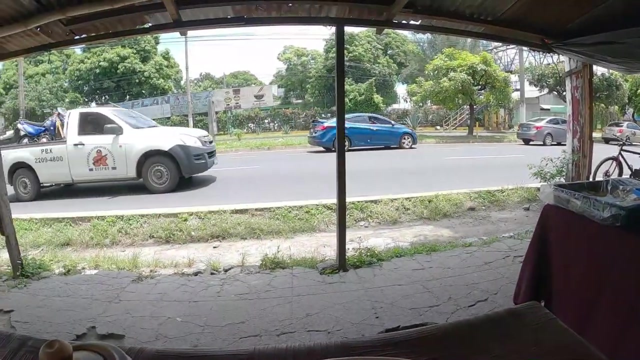 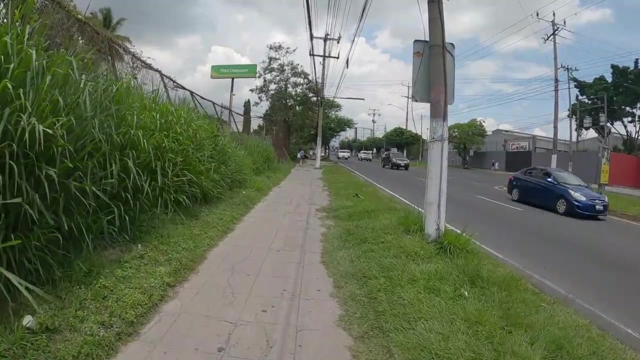 Hopefully we can run into a Walmart. If not, Then I'll try to flag down a taxi And do the best I can to communicate, Taking me to the Airbnb or Walmart. so we'll see. Alright, guys, I left them a decent tip. They were trying to run me down and give it back to me. 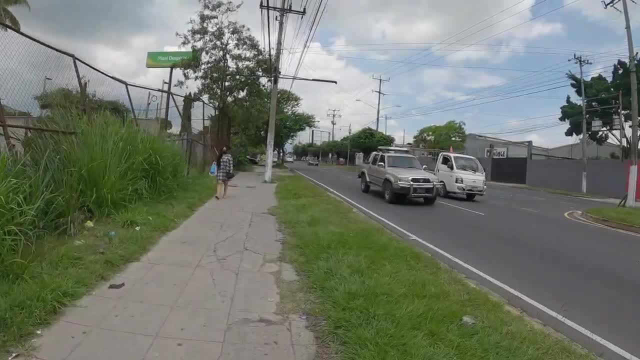 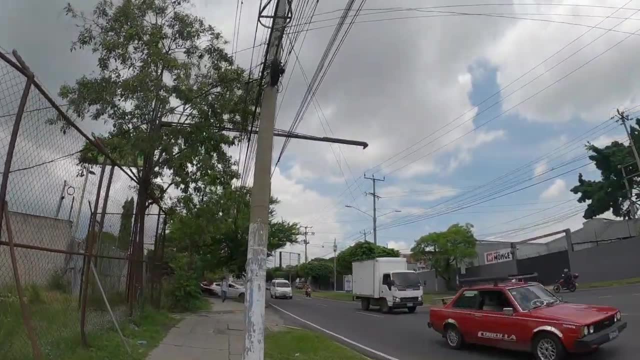 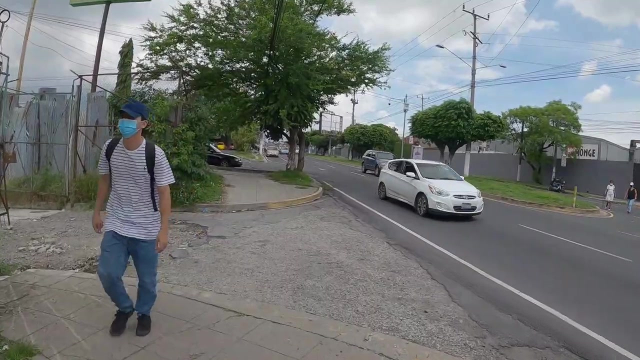 I was like: no, it's for you Such a wholesome moment. Alright, we're back on the grind and, oh my gosh, Started walking and I feel a cool breeze, As if it's about to start raining. Then also, I see another hill up here: Buenas. 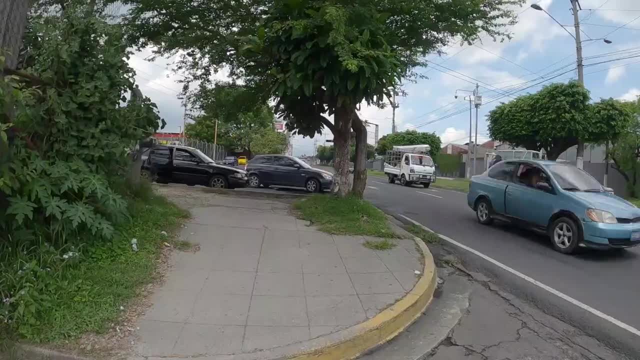 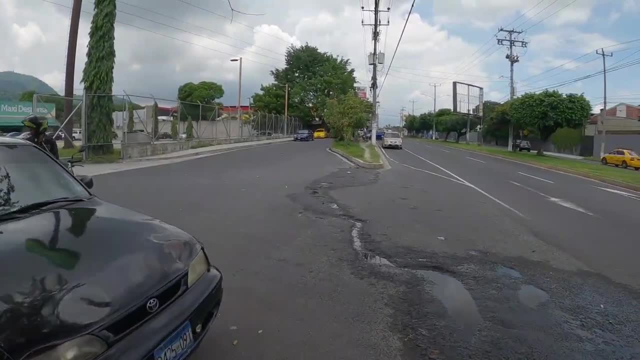 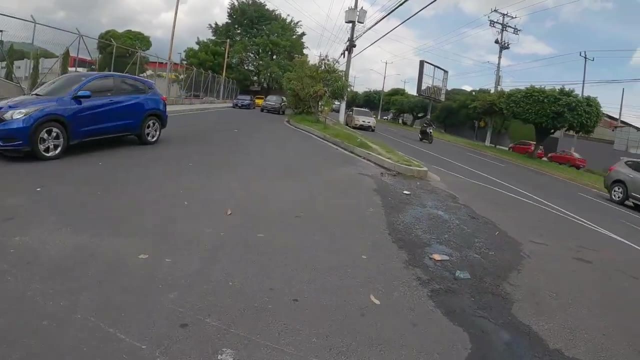 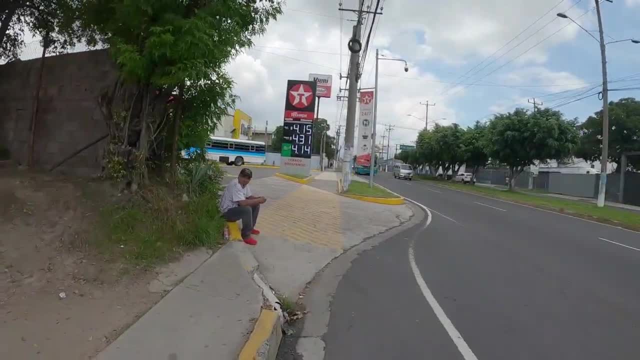 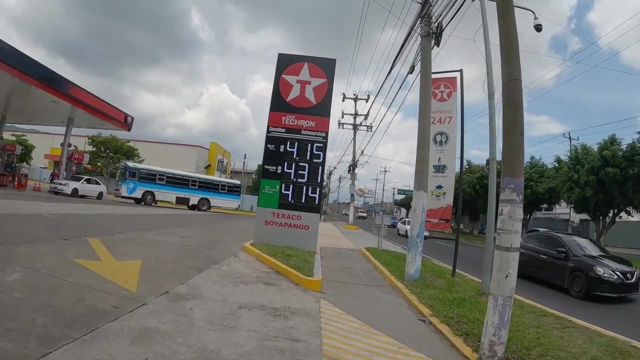 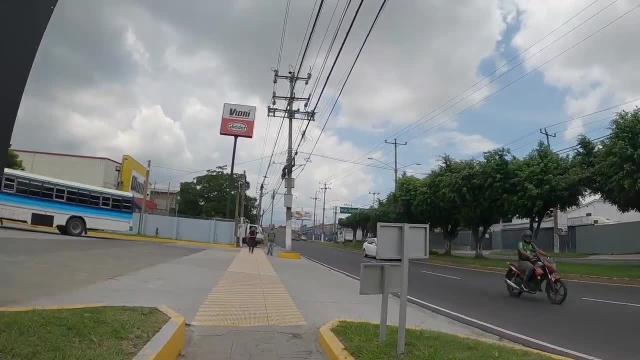 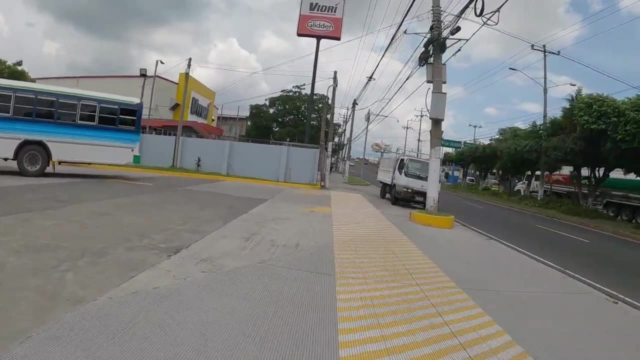 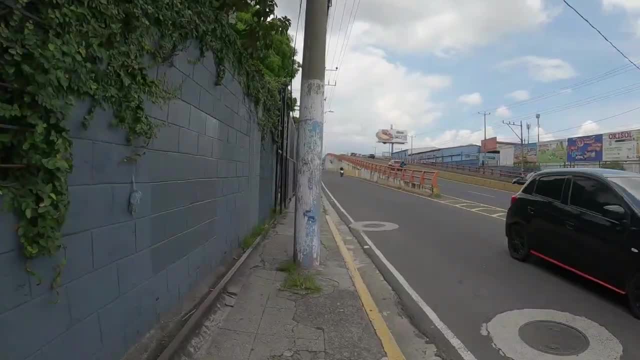 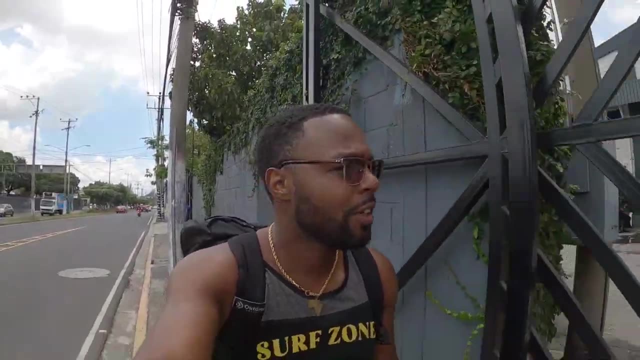 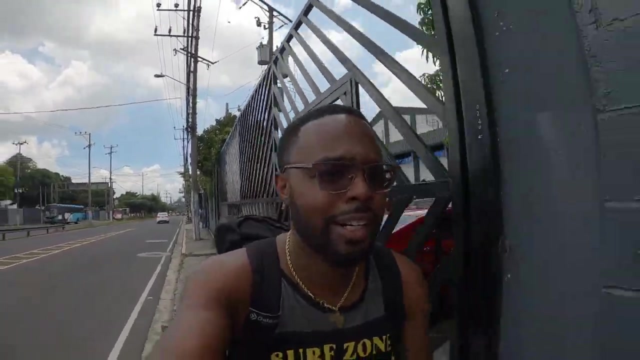 So what are you guys' opinion of El Salvador thus far, Based on the videos that you've seen? Somebody talk to me- right now I don't have anyone to talk to. No, I'm joking, No, but seriously, what do you guys think about El Salvador? 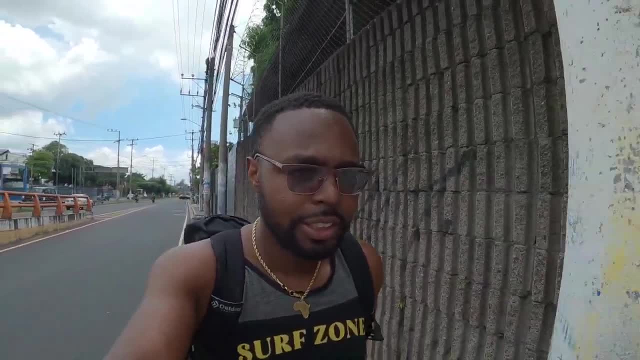 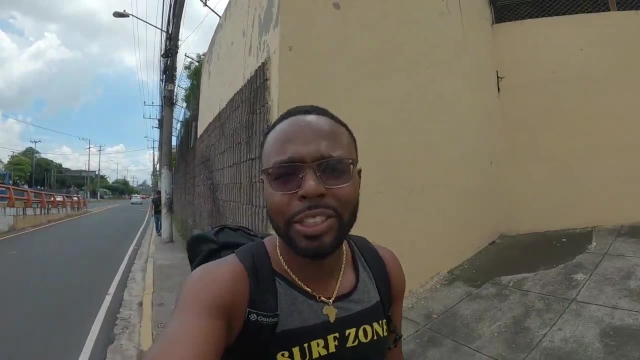 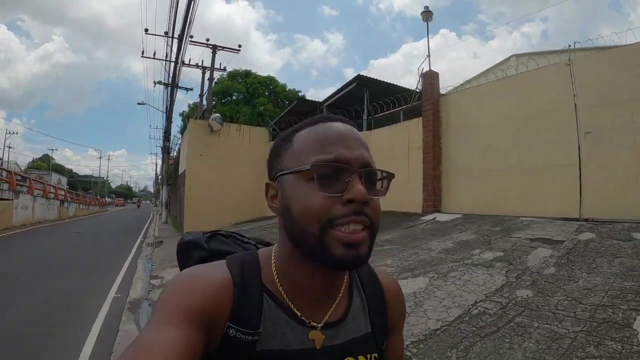 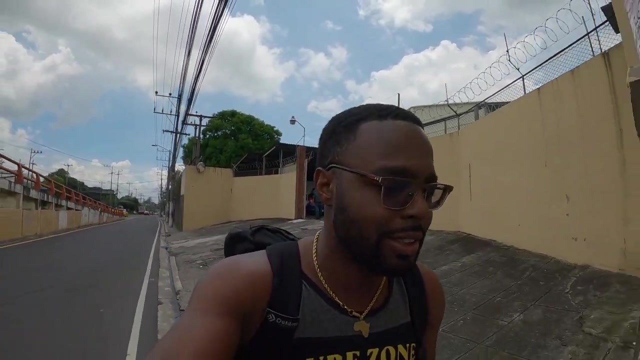 From the videos that I've posted. do you see yourself coming Visiting? Do you think you can add it to your vacation list? I'm telling you right now. Right now is the best time to visit El Salvador, Because within the next 5 to 10 years it is going to be a very hot tourist destination. 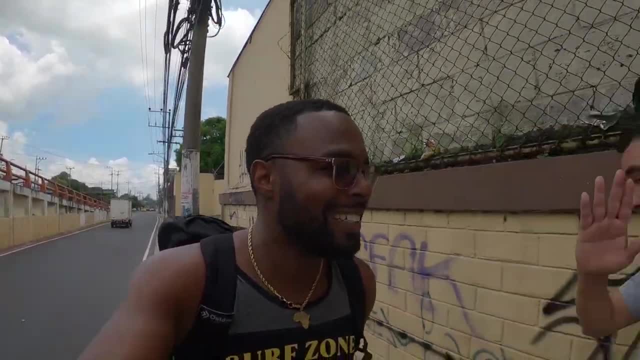 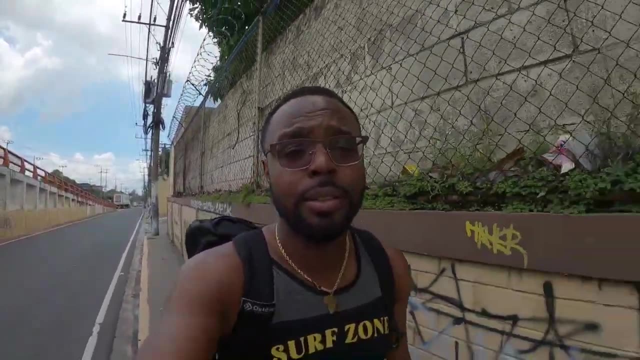 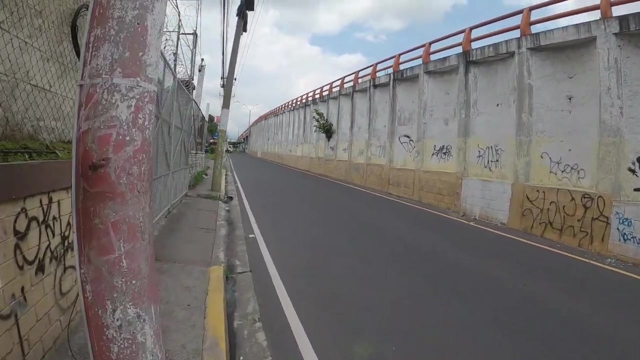 Similar to that of the Dominican Republic, Similar to the Dominican Republic in some places in Mexico. I'm sorry, I'm telling you They're not playing. They're really, really growing. Okay, I look like we have another bus stop up here. 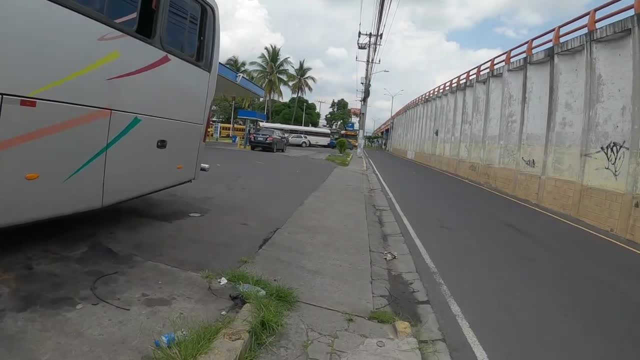 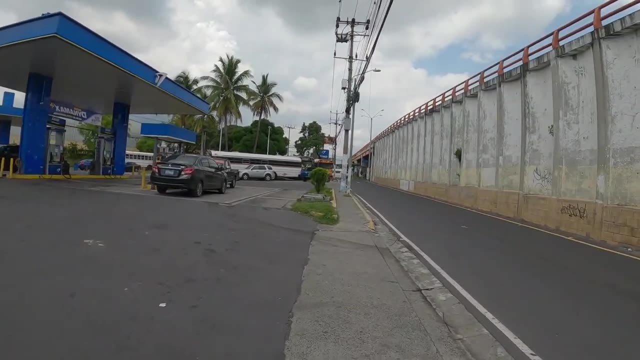 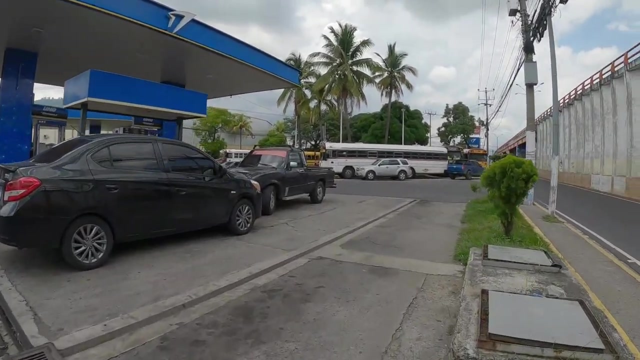 Alright, Alright, I'm going to put the camera away until I can find a taxi, Or if I can get a random, Or if I can get a random signal to come and spook your boy up. Alright, guys, see you in a second. 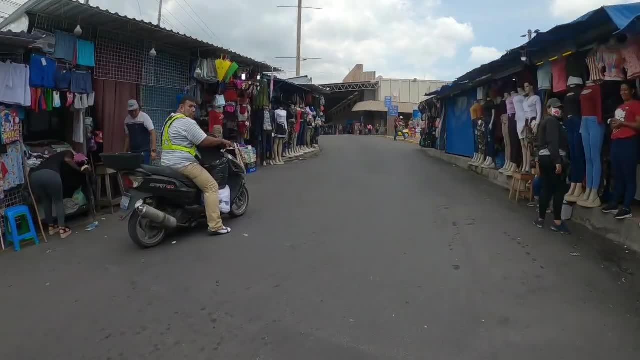 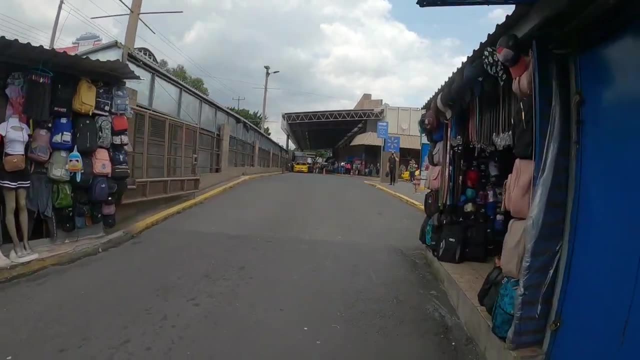 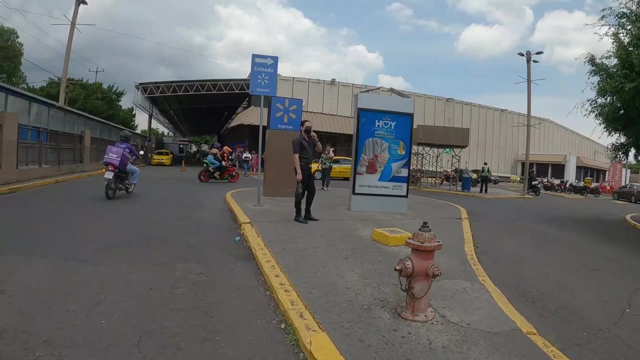 So, number one: just walk in the streets of San Salvador, feel completely safe. But then, number two, I just literally randomly stumbled upon a Walmart. We want to talk about luck. just a random draw on the hat. I just look up and see the Walmart sign. 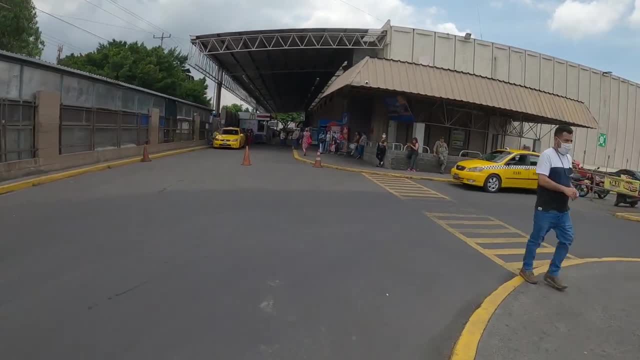 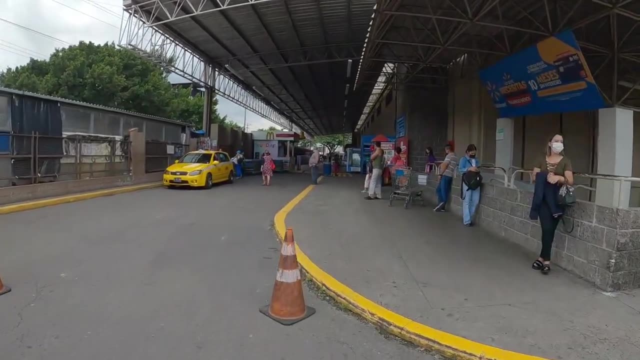 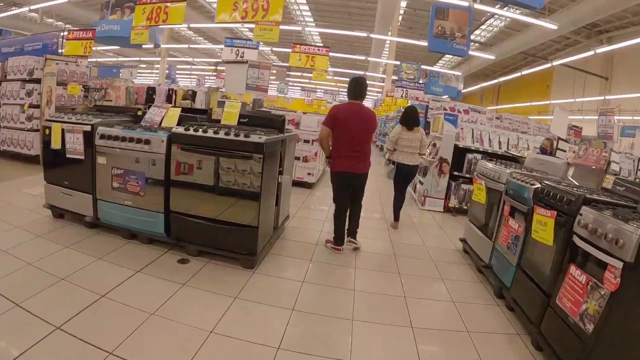 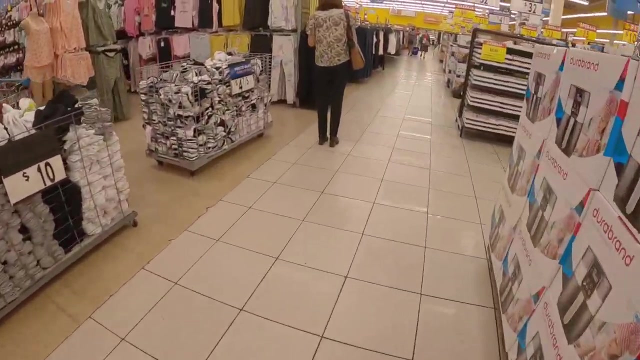 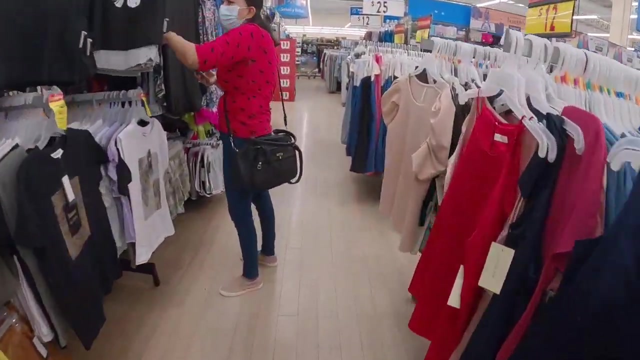 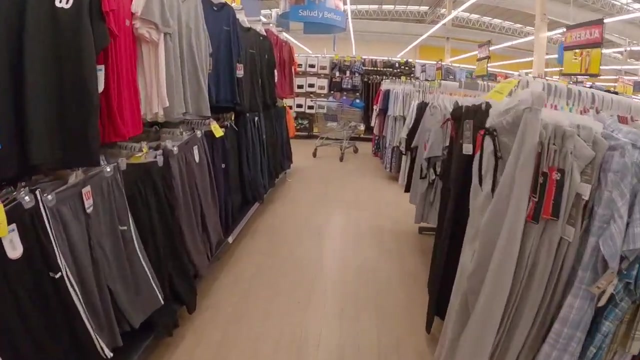 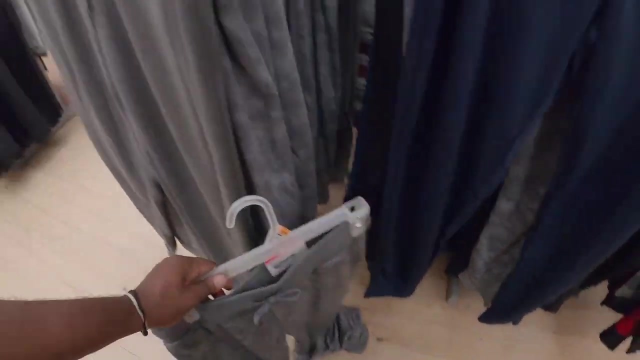 So Then there's multiple taxis out here. Guys, I think that's a dub. I think that's a dub. Welcome to Walmart in El Salvador. Very clean, See, I got it all. Centro de Bebe. Oh, sorry, I dropped something. 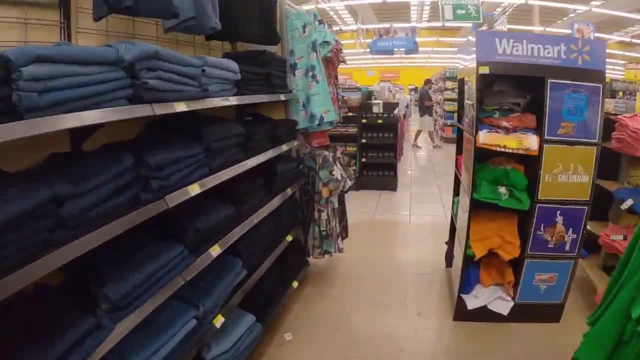 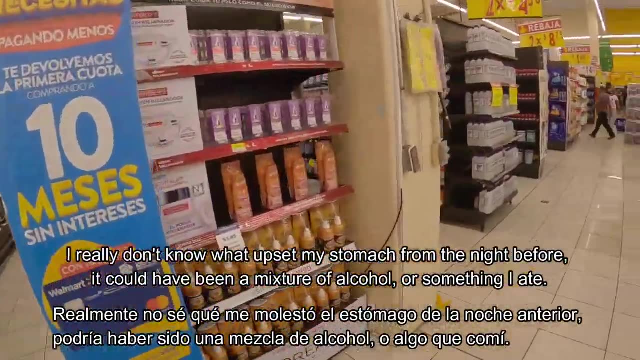 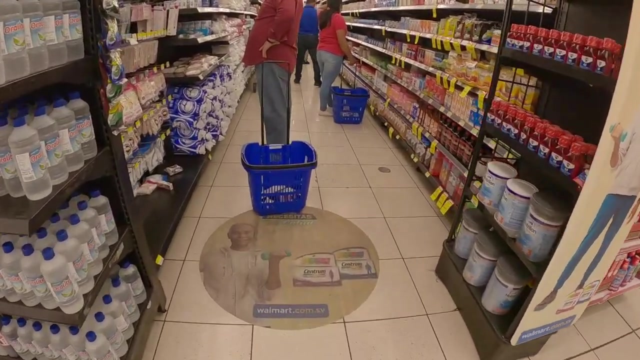 Alright, guys, I'll be completely honest with you. The reason I'm in Walmart right now is because I think I accidentally drunk some of the local water and it kind of messed me up a little bit. so i'm here looking for a remedy. 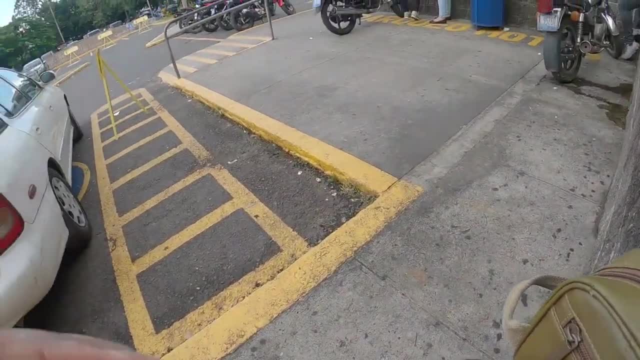 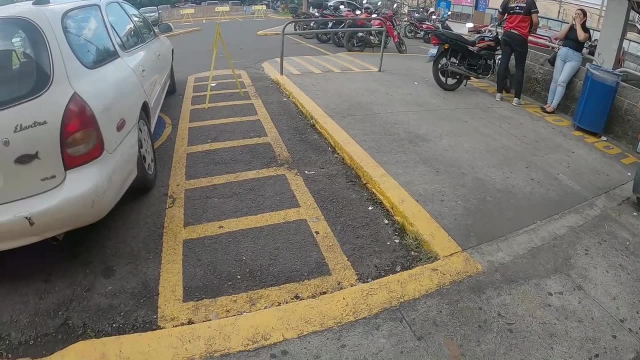 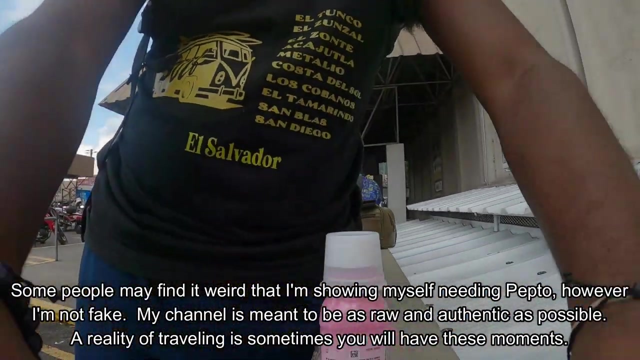 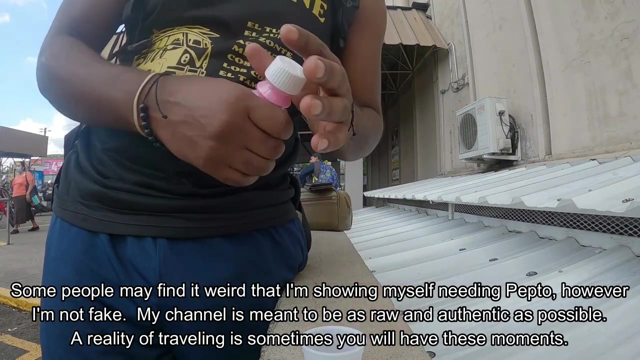 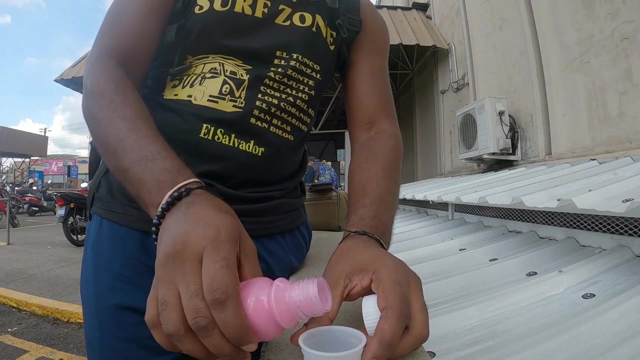 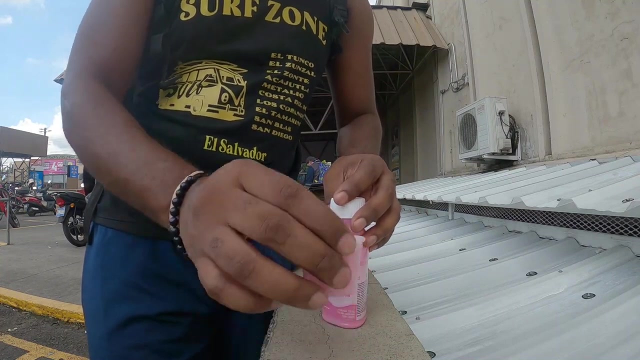 all right, guys, this is the moment that i've been waiting for. i've needed this. oh crap, okay, all right. i think i'm supposed to take 30 millimeters if i read that. right, all right, gotta take it to the head. you're gonna take it to the heat. 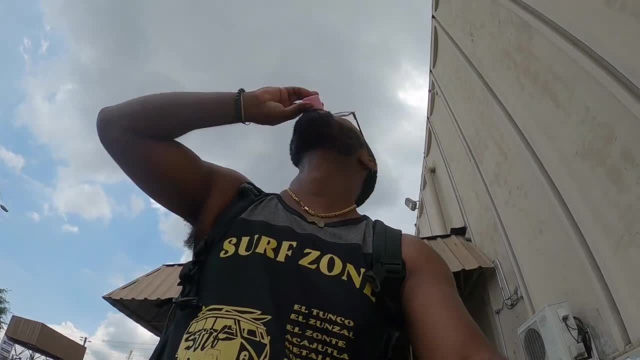 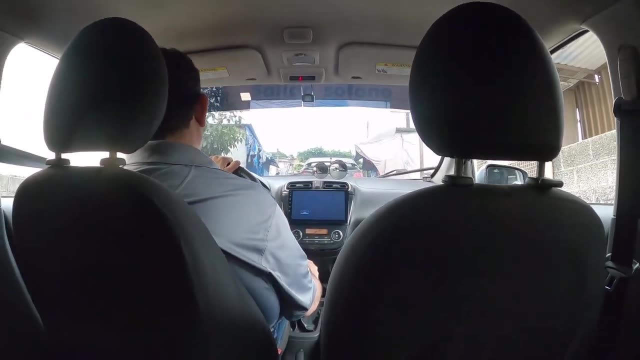 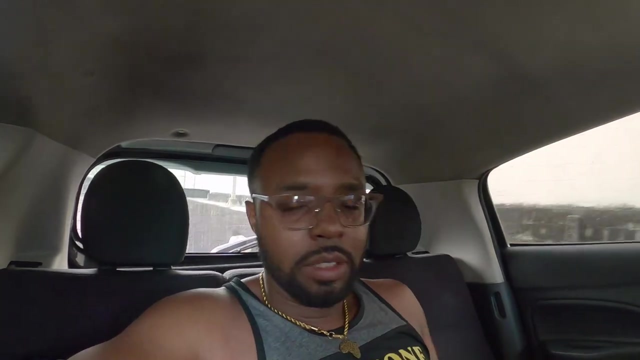 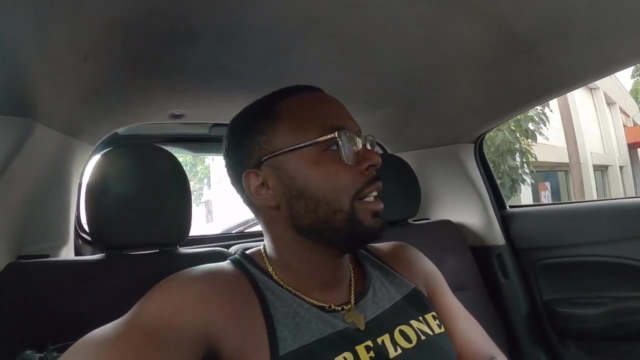 hmm, i hope that helps all right guys. so i was able to, uh, finally, uh, um, get a little bit of signal, so i made sure i stayed still on my phone caught up to it, and then i was able to order an uber, so finishing the trip to san salvo right now. 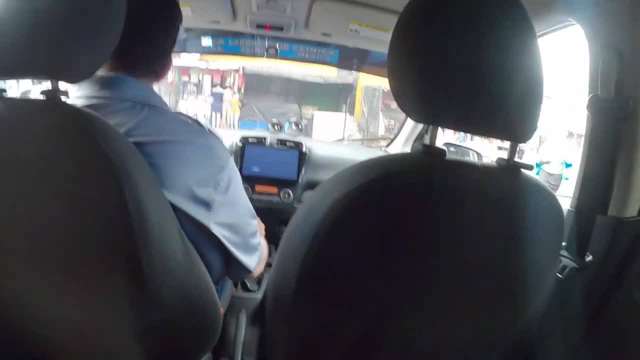 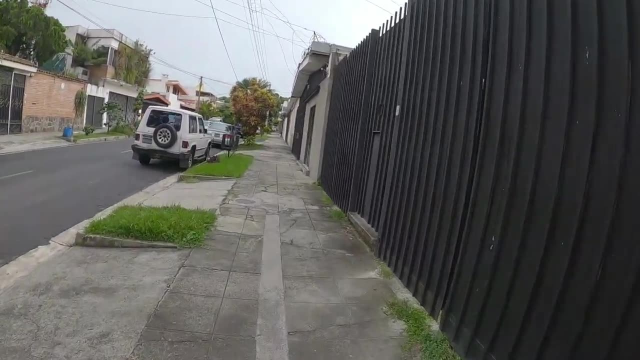 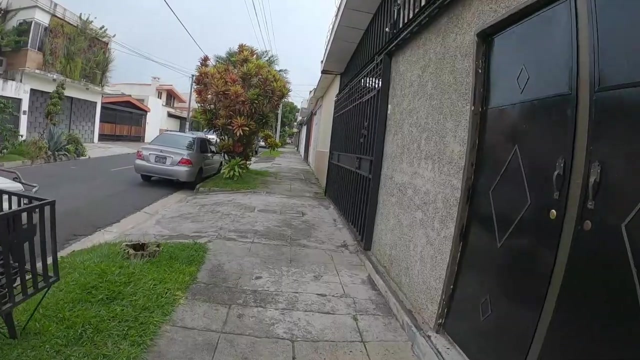 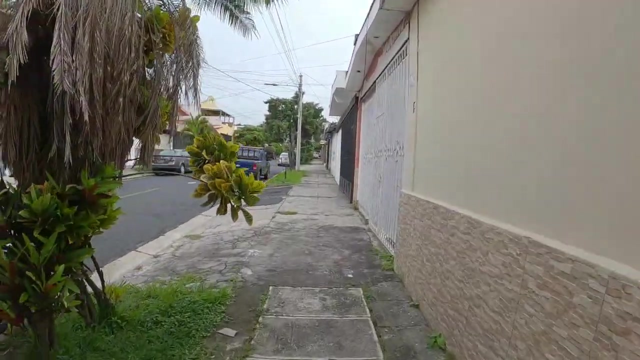 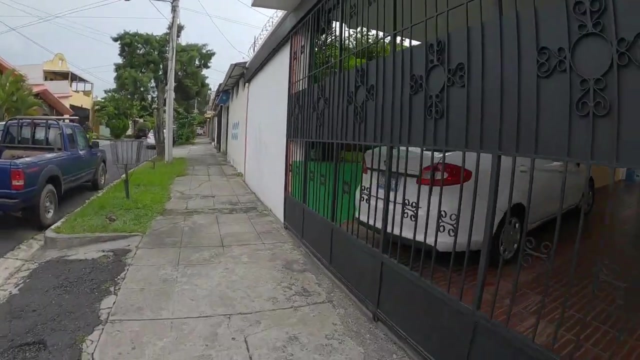 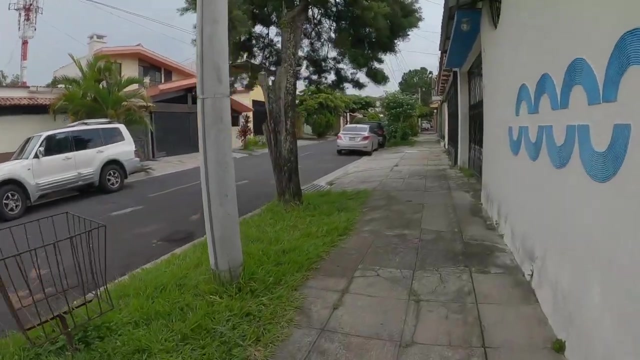 and then we can get the day started. i'll be completely honest, man, there's some. i've seen some really nice houses here, both in san salvador and in suchitito or suchitoto. my bad got the ford focus there, got the ford ranger. is that salvador a ford company? any ford country? 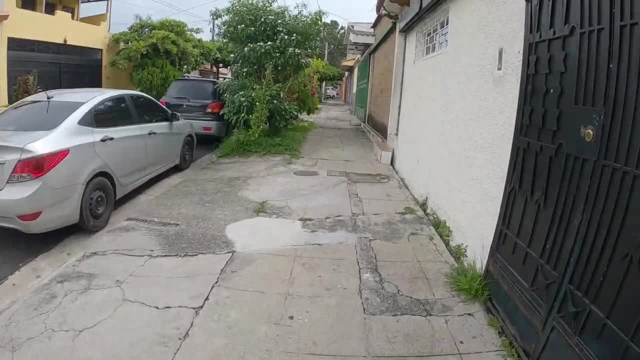 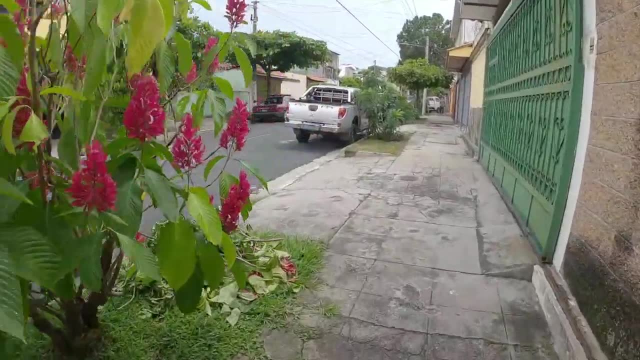 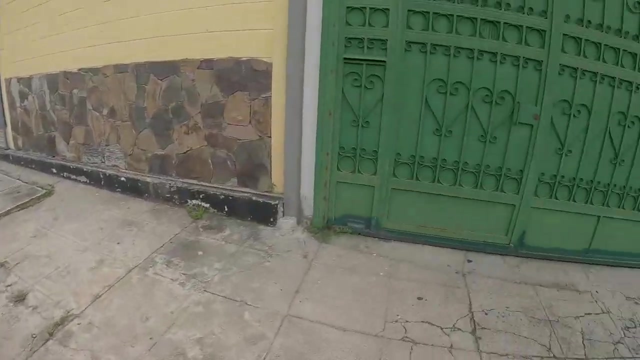 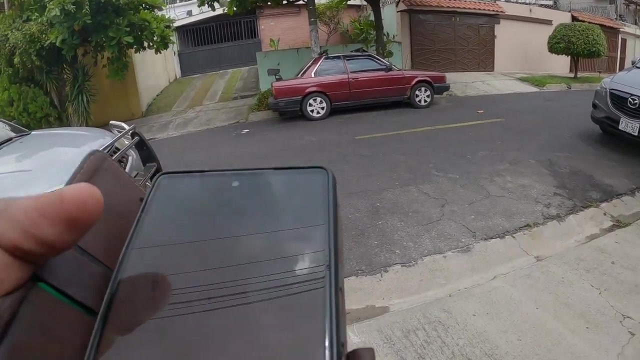 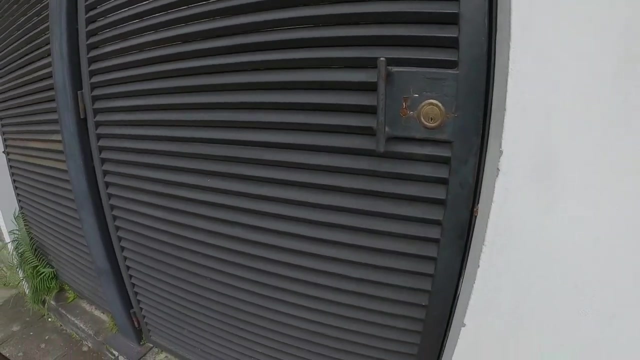 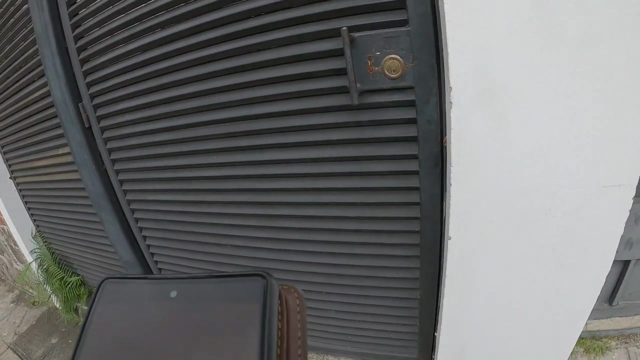 whatever they're eating over there, it's almost divine. all right, guys. so it says that my airbnb should be right here somewhere. all right, let's see right here somewhere. all right, let's see where they're at all right. 26b- all right, i'm here. would it already be open? no, all right, let's see once i get here.